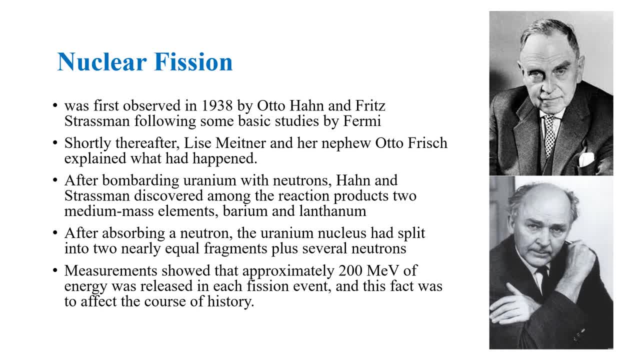 a German chemist, and Fritz Strassmann, a German physicist, following some basic studies by Fermi. This was observed again in 1938, when the Germans, led by Adolf Hitler, was busy convincing the world of the superiority of the Germans. This was during the World War II. 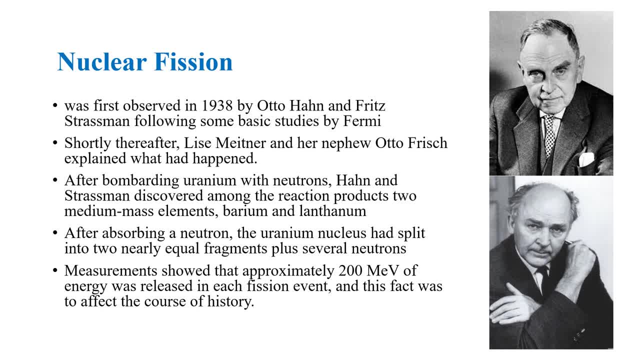 Shortly thereafter, Lis Mitter and her nephew Otto Frisch explained what had happened. They found that after bombarding uranium with neutrons, Hahn and Strassmann discovered among the reaction products two medium-massed elements, barium and lanthanum, And after 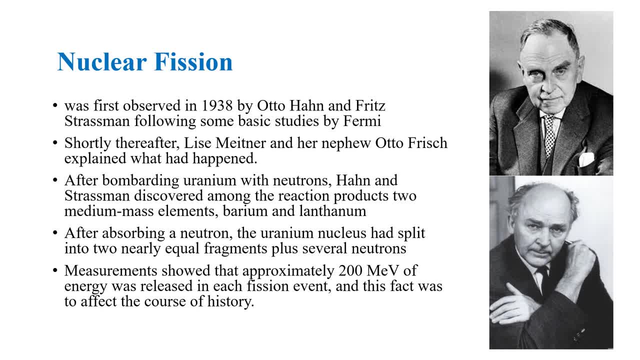 absorbing a neutron, the uranium nucleus had split it into two nearly equal fragments plus several neutrons. These measurements are explained by the liquid drop model. Measurements showed that approximately 200 MegaElectionVolt of energy was released in a recent report on the German study of the power of a neutron. The measurement that I found was 약2mEVvEV. 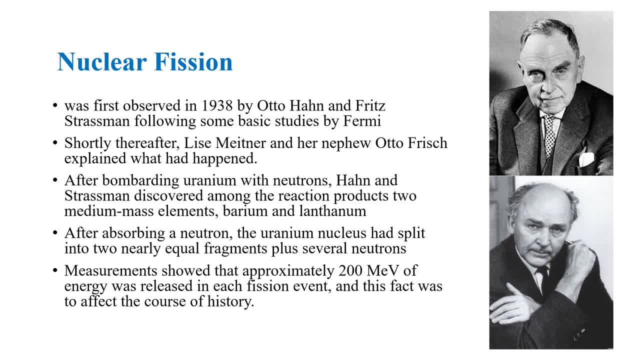 efficient event and this fact was to affect the course of the history. so after this discovery, the german nazis, or the german government or the nazi government, actually started research about this one. as you can see, it can produce 200 mega electron volt of energy, which can actually 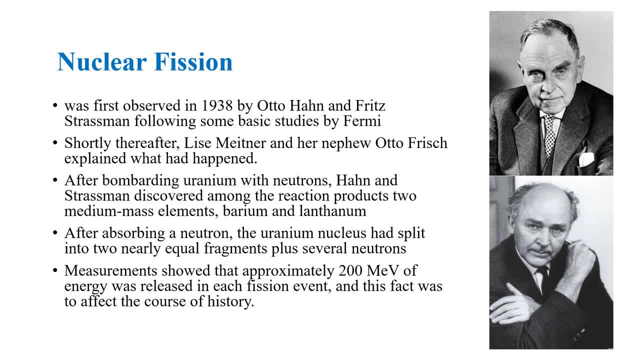 use which can actually be used in the war. and then albert einstein found out about this and wrote a letter to president roosevelt about the dangers of nuclear fission, and from that started the manhattan project, which made the first nuclear bomb, which was first dropped in hiroshima, and 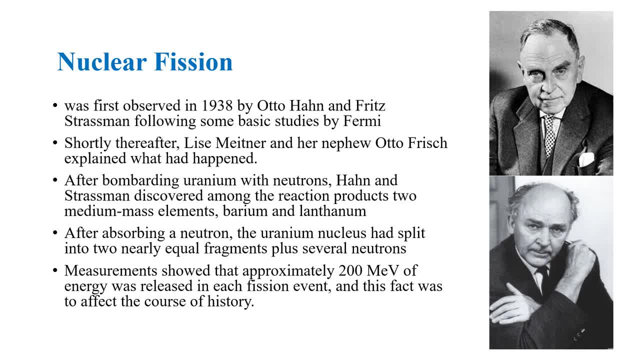 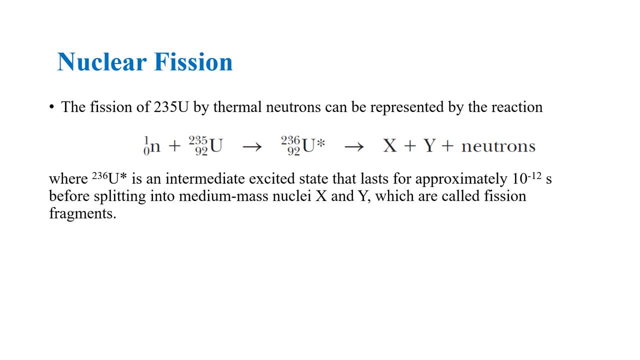 nagasaki, which then ended the world war ii. the fission of uranium-235 by thermal neutrons can be represented by the reaction given below. what you have here is a stray neutron that needs uranium-235 or is absorbed by uranium-235, which then forms an unstable uranium-236. 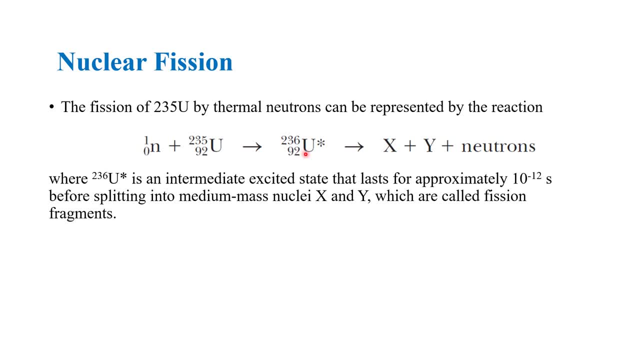 And since this is an intermediate excited state or unstable state, this lasts for approximately only 10 to the negative 12 seconds only, before splitting into your medium mass nuclei X and Y, which are what you call your fission prevalence, and also produce other extra neutrons in the 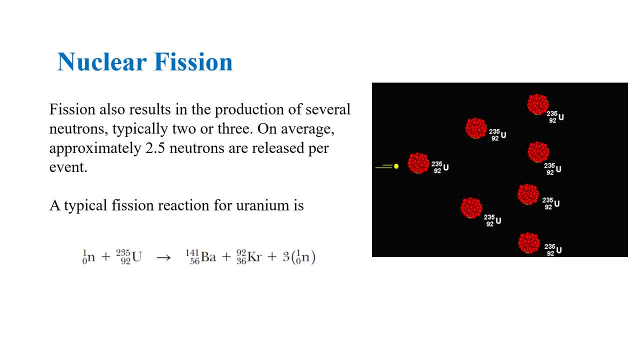 process. Fission also results in the production of several neutrons, typically two or three, and on the average approximately 2.5 neutrons are released per event. As you have seen in the previous slide on the representation of the process of nuclear fission, there are extra 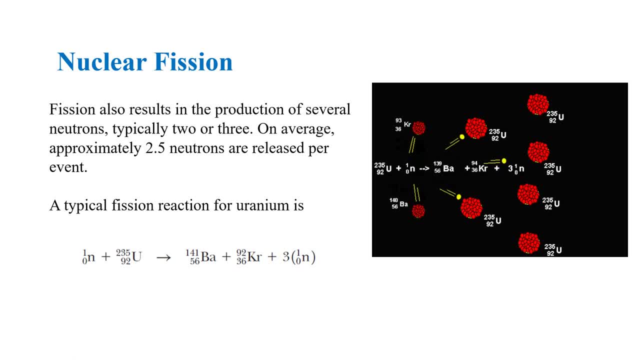 neutrons that are produced in the fission process. For example, you have a typical fission reaction for uranium, given below. You have a strain of 1 neutron, or just 1 neutron that hits a uranium-235 nucleus And since this is absorbed, 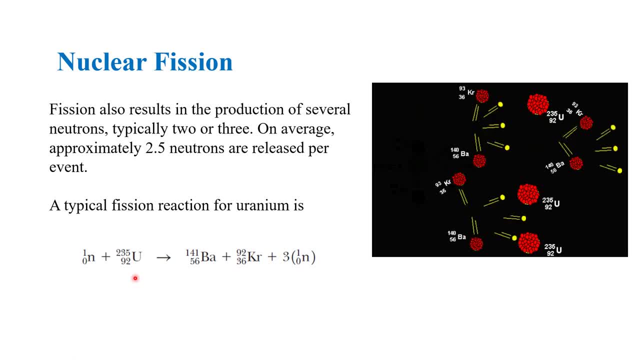 it produces again an unstable uranium-236, which then splits into your barium-141 and krypton-92.. And this process produces around 3 neutrons And, as you can see here in the figure, this just is one neutron hitting your uranium-235,, but these other neutrons that were created on the process 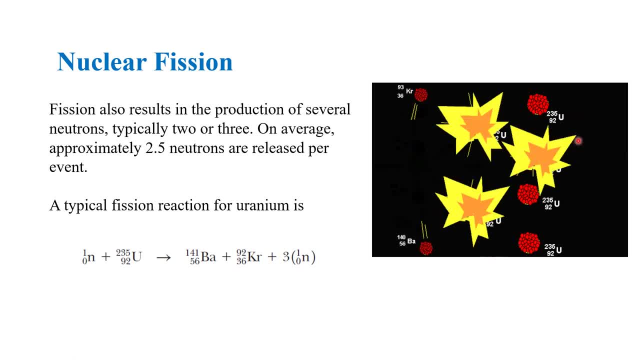 actually hits other neutrons, around your chamber for example, which then triggers a chain reaction. This chain reaction in your nuclear fission is what creates the power, which is 200 times the power of the- of the initiating neutron, And this is the power of the nuclear fission reaction. 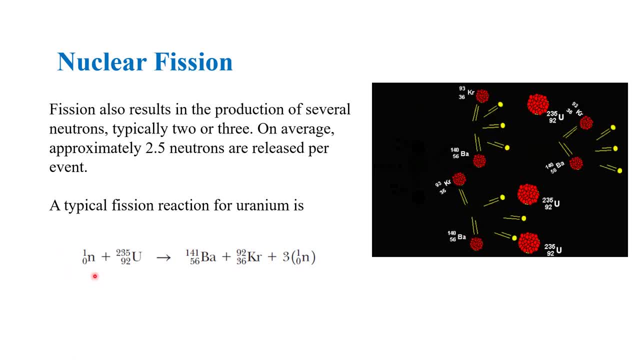 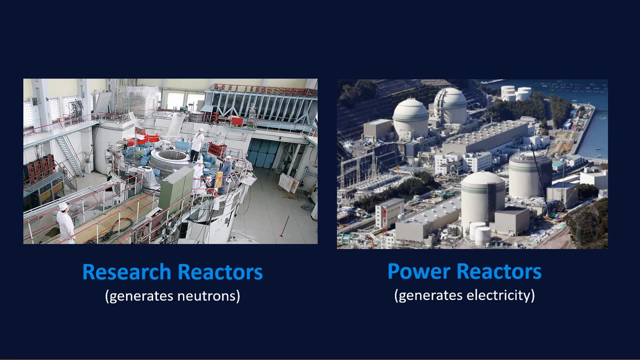 And this is the power of the initiating neutron, which is this one here which creates very large or massive power which can be used in your nuclear reactors or even also in nuclear bombs. We have two types of nuclear reactors. The first one is your research reactors, which generates 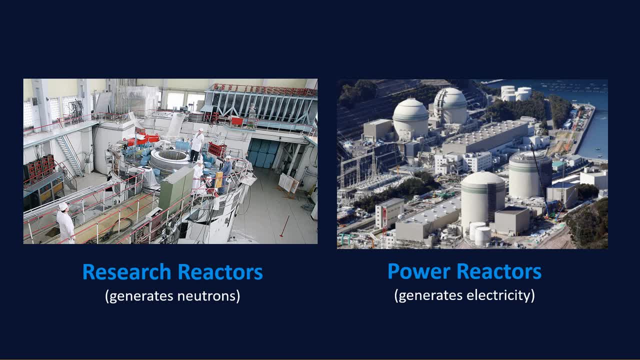 neutrons for the use of research, in medicine, in agriculture and etc. The second type is your power reactors, which generates electricity, And for this lesson we are going to focus on your power reactors, the one that is more commonly known as your nuclear power reactors, or your NPP or NPR. 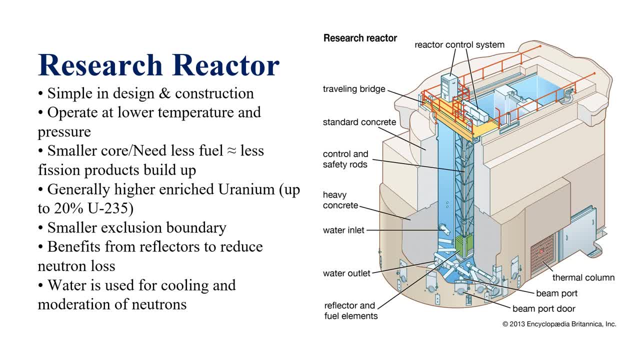 But let's define first what a research reactor is. So typically, an image is an example of a research reactor which is simple in design and construction. We actually have a research reactor in the Philippines and this is located in. this is located in the Philippine Nuclear Research Institute. Okay, and you can view it. 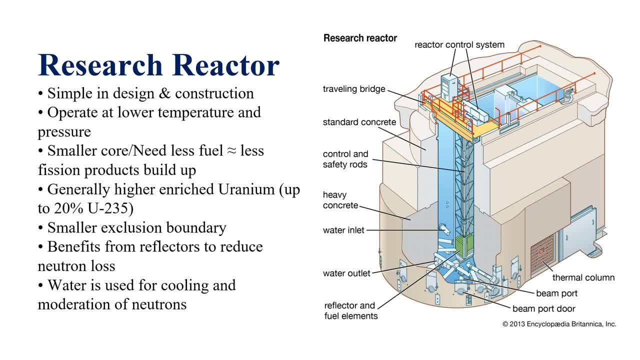 in the internet how it looks like, But typically it just looks like an egg outside that you have a research reactor inside of it. It operates at lower temperature and pressure and it needs a smaller core, which means it needs less fuel, But this also produces less. 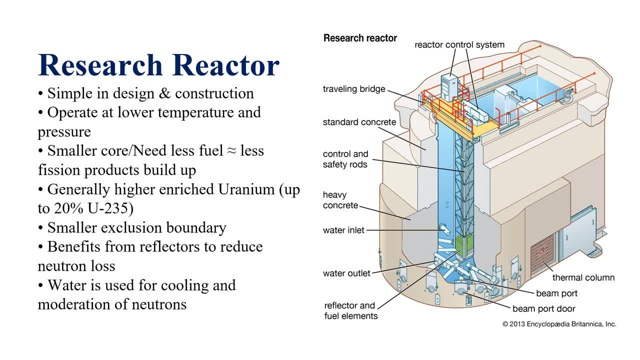 efficient products to build up And generally higher enriched uranium. up to 20% uranium-235 is used in your research reactors. This has smaller exclusion boundary as compared to your power reactors, but has benefits from reflectors to reduce your neutron loss And for your research. 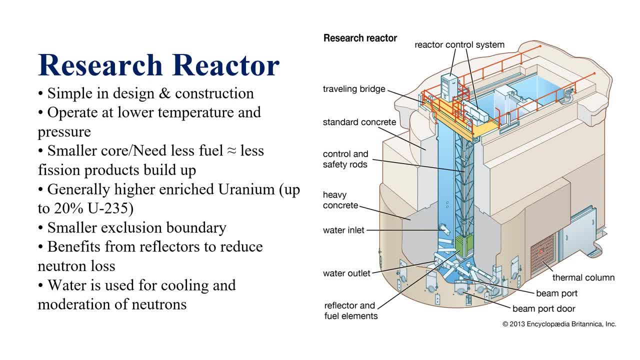 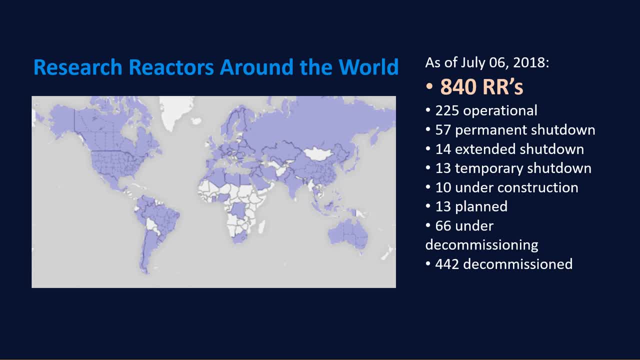 reactor water is used for cooling and moderation of your neutrons. As of July 6, 2018, we have around 840 research reactors that were built around the world, but only 225 of this one is operational and 57 are in permanent shutdown. For King is an extended 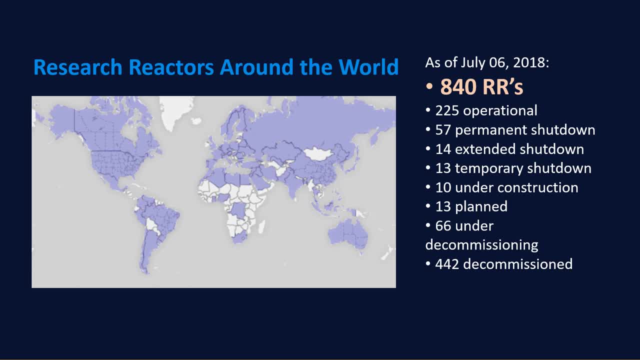 shutdown including the PRR-1,, which is the Philippine Research Reactor in the Philippine Nuclear Research Institute. So we actually have a research reactor in the Philippines. It's again called your PRR-1, but it's not in use. It's in extended shutdown, but there are plans to revive this one. 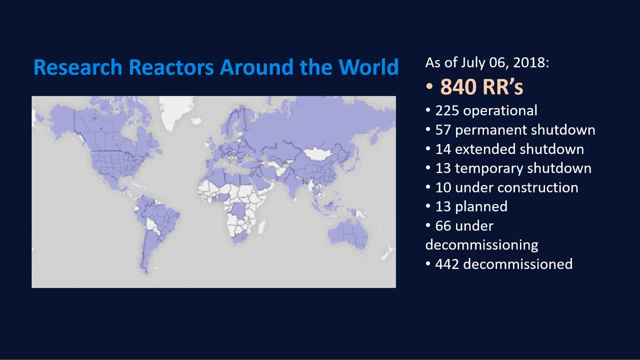 or to commission it again, which is called your SATR plan, And we're going to discuss more about the SATR plan in the next lessons. 10 are under construction, 13 are planned and 66 under decommissioning, and 442 are decommissioned. Decommissioned meaning it's not anymore used. 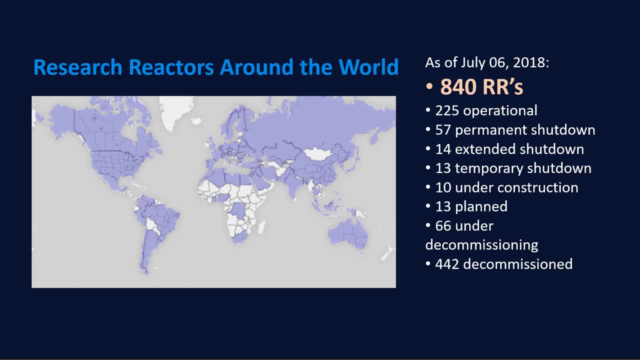 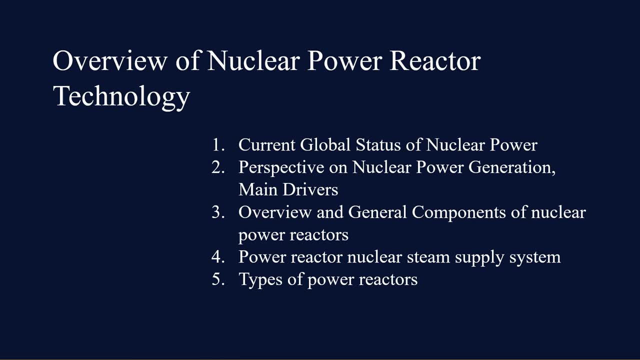 and will not be used anymore. So, as I've said, in this lesson we are going to discuss more about your power reactors and we'll have a brief overview of the nuclear power reactor technology. We are going to discuss the current global status of nuclear power, the perspective of 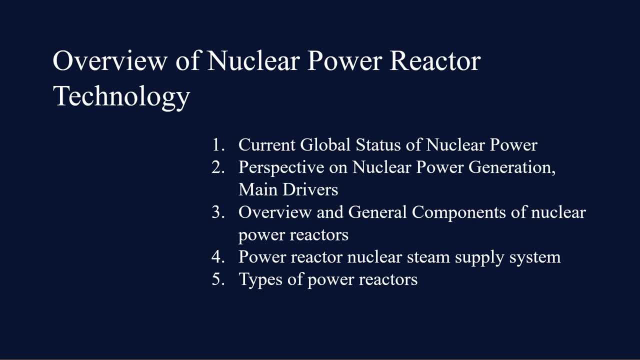 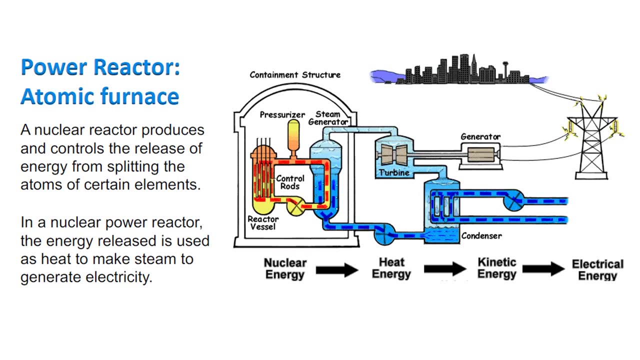 nuclear power generation main drivers and the overview and general components of nuclear power reactors. And we're going to discuss also the power reactor nuclear steam supply system and also the types of your power reactors. So what's a power reactor? A power reactor is also 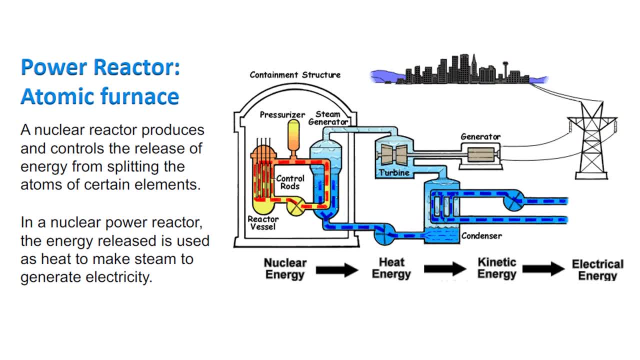 called an atomic furnace. So a power reactor is a nuclear reactor that produces and controls their nuclear power, And it's a nuclear reactor that produces and controls their nuclear power. And it's a nuclear reactor that produces and controls their nuclear power And it also produces. 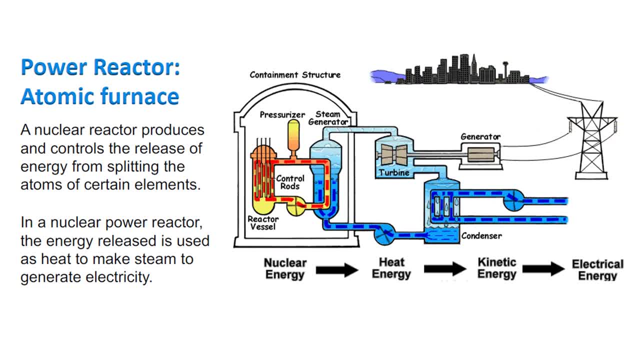 the energy from the atoms of certain elements, Let's say, for example, of course, your uranium-235.. In a nuclear power reactor the energy release is used as heat, to make steam, to generate electricity. So it's just actually the same as your fossil fuel plant or your full power plant. So the energy 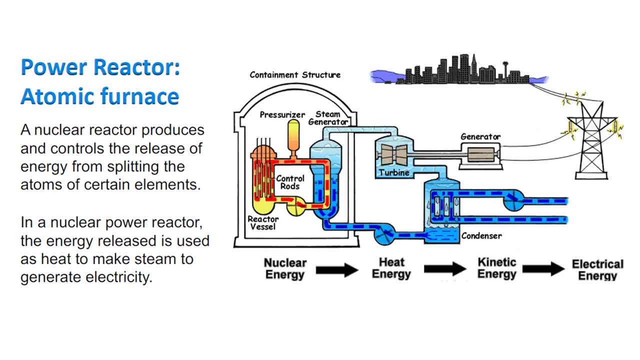 release is used to boil water, to make steam. And this steam, here generated from the boiling of the water, will be used to power up your turbine. and when this turbine is powered up it will move your generator and, by electromagnetic induction, will create electricity powering up your cities or your homes. so from your nuclear energy you produce your heat energy. 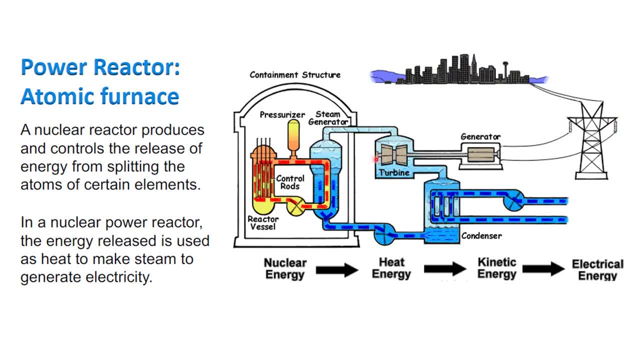 in the form of your steam, and the steam will, the kinetic energy of your steam will be used to to move your turbine, which then is transformed into electrical energy via your generator. so it uses a lot of thermodynamics and electromagnetism in in just producing your, in your power, in your 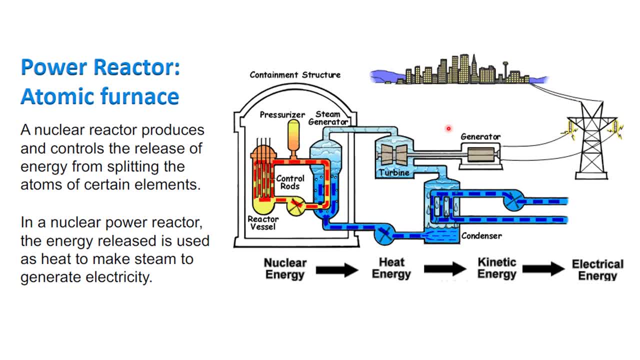 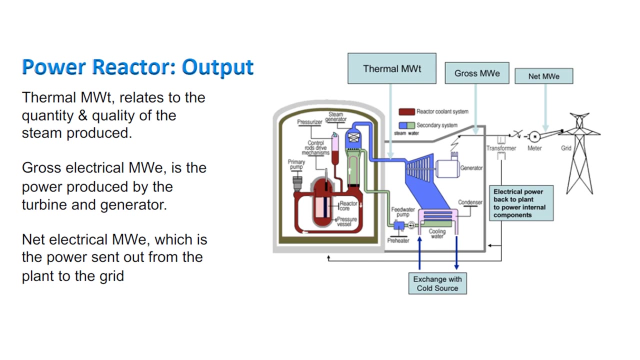 nuclear reactor. but again, this is, it's the same process with um, your fossil fuel, or your core coal power plants, which uh uses heat energy to form steam in order to drive your turbine. mat experience. let's discuss the different outputs in your power reactor. one is your thermal mwt or your 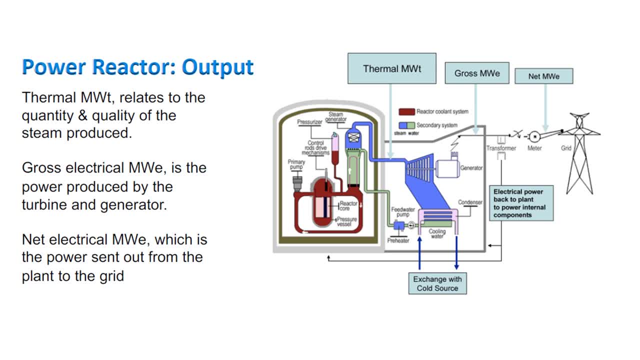 megawatt thermal. this relates to the quantity and quality of the steam produce. and we also have your gross electrical mega megawatt electric, which is the power produced by the turbine and your generator, your net electrical megawatt electric, which case the power is sent out from the plant to the grid. 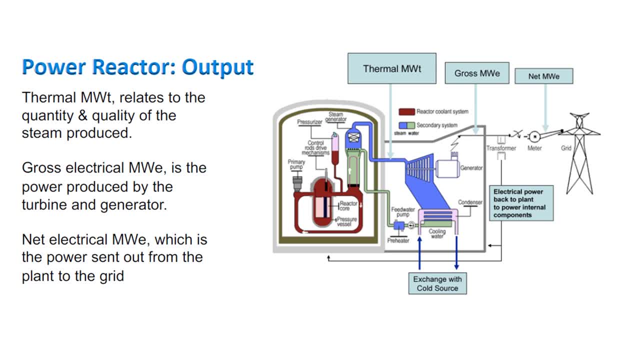 what is actually important here is your net electrical, or your net electrical megawatt electric, because this is the actual energy that we are going to use, uh, in powering up your neighborhood. so this is again the power sent out from the plant to towards the degree so you have. 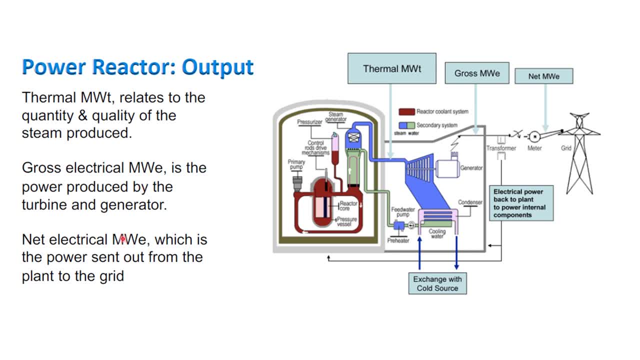 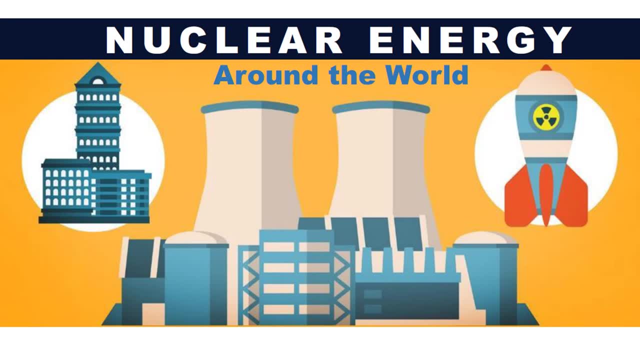 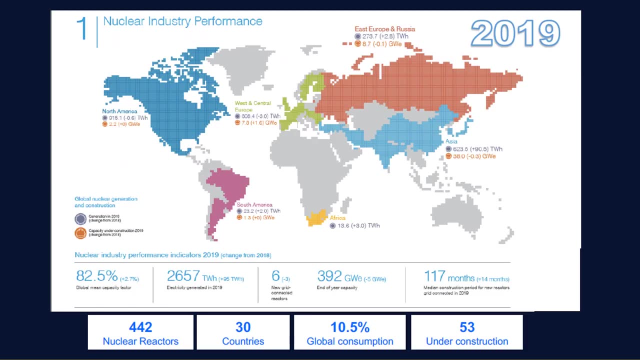 your megawatts thermal, your gross electrical megawatt electric and then your net electrical megawatt electric. let's look at the overview of your nuclear energy around the world. so this is a map of the world of the nuclear industry performance in 2019. 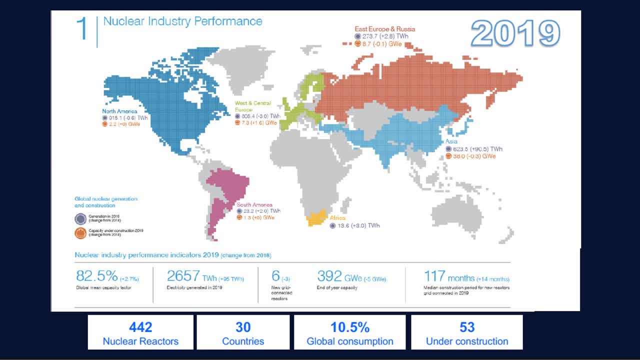 and we have around 442 nuclear reactors around the world, uh, which is divided into 30 countries, and we have 53 under construction, but of course we do not have one here in the philippines, so we do not have a nuclear power plant here. most of the nuclear 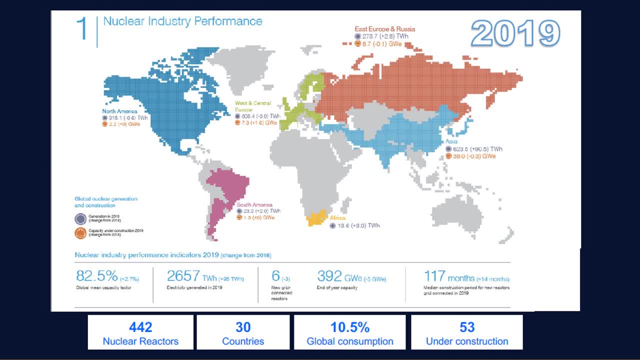 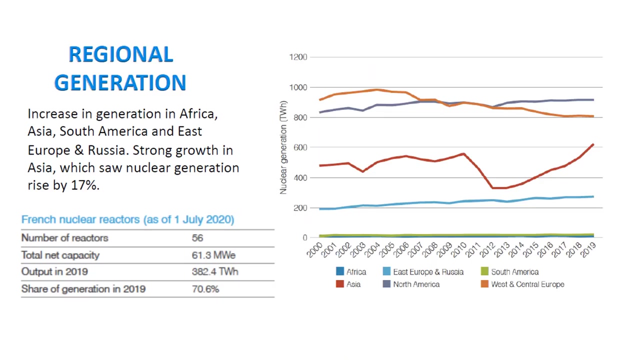 reactors are in france, which actually powers up 70 percent of their or of their energy. so also we have an increasing interest of using nuclear power plants in asia, specifically in china and south korea. this is the regional generation. there's an increase in generation in africa, asia, south america and east europe and russia and 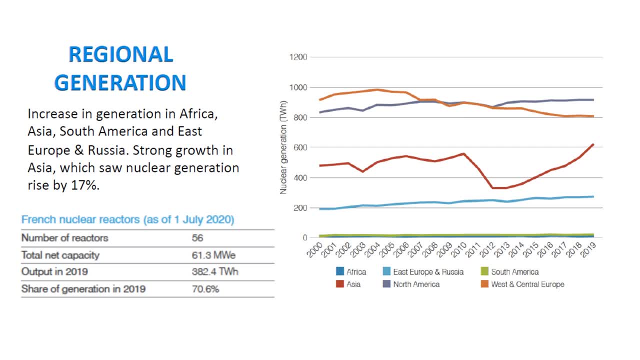 there's a strong growth in asia, which saw nuclear generation rise by 17. as i have said earlier, there is a strong increase of uh nuclear interests in asia, specifically in china and south korea. this one here is uh. this graph here is for asia and, however, there is a decrease in interest from 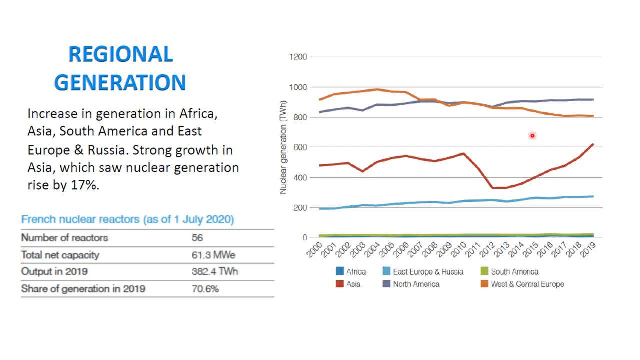 the west and the central europe. so most of the reactors now are in uh are in france and we have at least 56 number of reactors in the french uh, french nuclear reactors, which produces um an output of around 382.4 uh terawatts per hour. 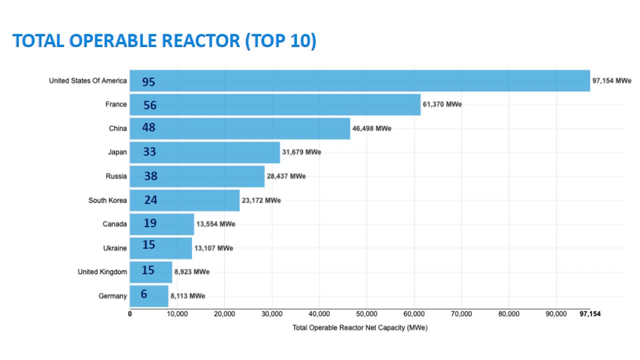 this already. top 10 total operable reactors: 95 are in the united states of america and 56 are in france, and we have 48 in china, 33 in japan, 38 in russia and we have 24 in south korea, 19 in. 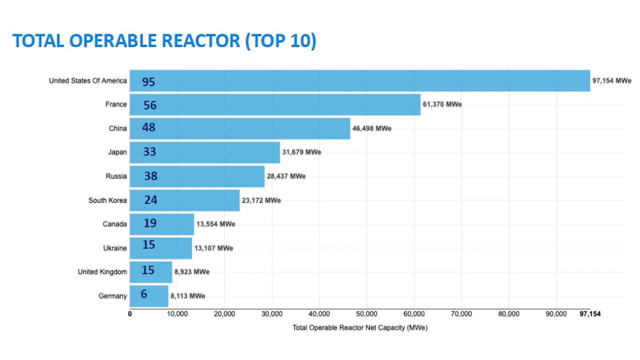 canada, 15, ukraine, 15 in united kingdom and we have only six in germany. germany is actually an interesting country to study- or imperial actors because, as you can see, it's a developed country, it's a first world country but, as you can see, they only use six per uh. they only have six. 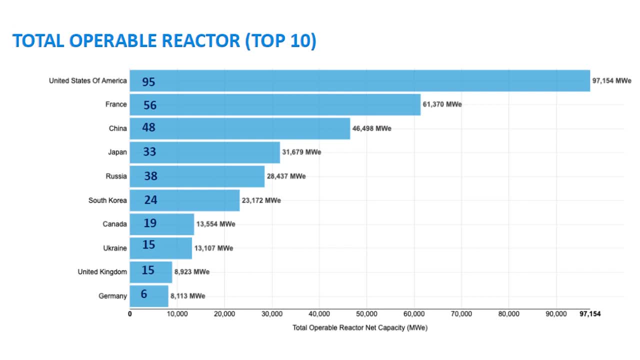 six operable nuclear reactors. There is this movement in Germany wherein they are planning to finally remove all these or stop using your nuclear reactors, which is in contrary to their claim that they wanted to remove anything, that any electricity generation which produces greenhouse gases. But, as you can see, nuclear energy is actually a clean energy, but Germany is trying to get. 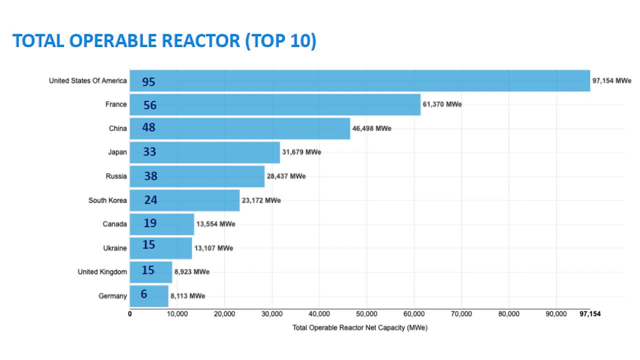 rid of it. So there's an interesting issue here in Germany when it comes to your nuclear reactors, And this is actually because of the various incidents like, say, for example, your Chernobyl incident and then of course also the Fukushima incident. 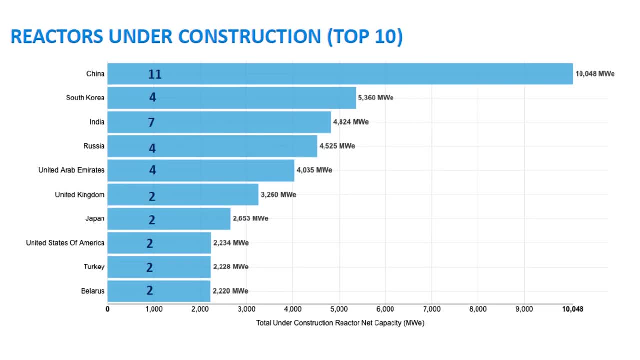 These are the top 10 reactors under construction. top 10 countries: You have 11 in China, 4 in South Korea and 7 in India, 4 in Russia, 4 in UAE, 2 in UK, 2 in Japan, 2 in United States, 2 in Turkey and 2 in Belarus. 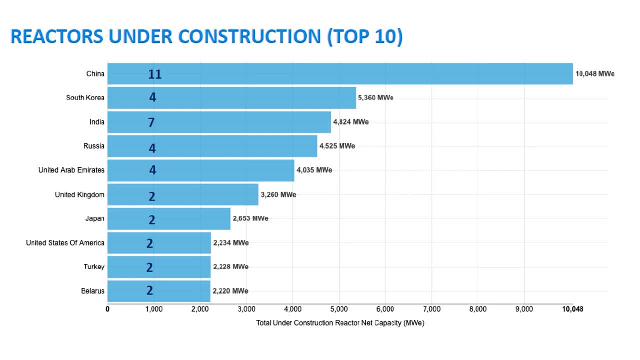 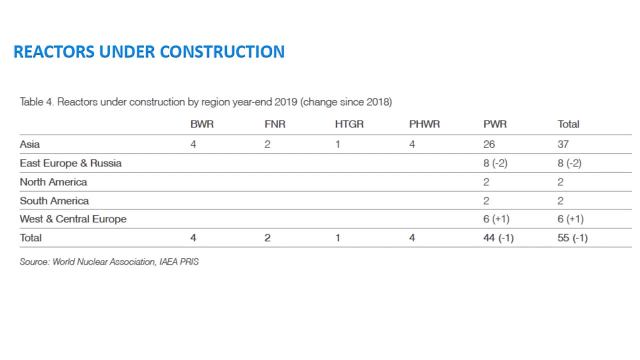 And, as you can see, among the top three, is found in Asia, which is in China and South Korea. So these are the breakdown of the reactors under construction. So for boiler water reactors in Asia, FNRA is top two And a total of 37 reactors are under construction in Asia and the rest are found in East Europe. 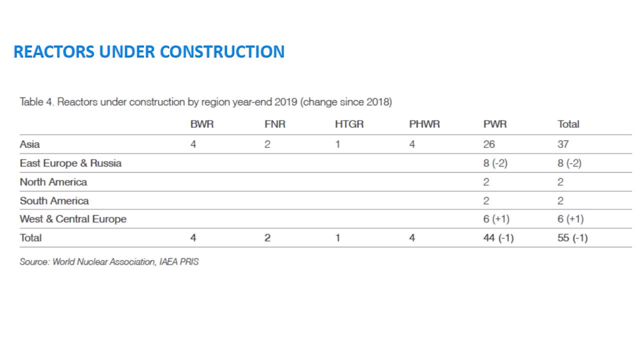 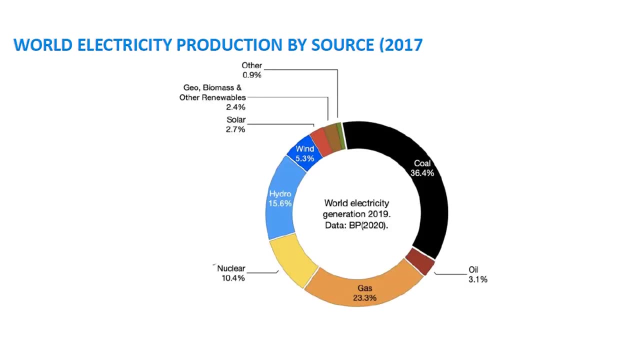 in Russia, North America, South America and West Central Europe. still no plants, of course, in the Philippines. And this is the world electricity production by source. As you can see, we still have 36.4% of our energy production which is dependent on coal. 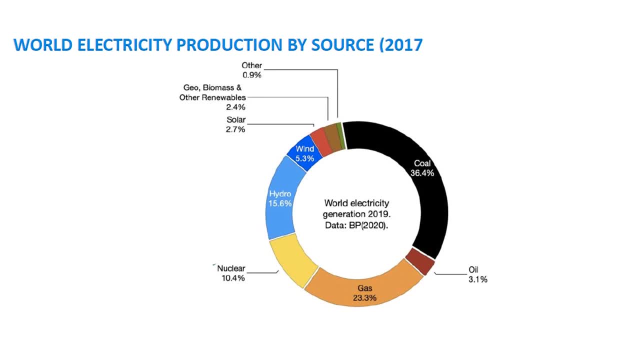 23.3% dependent on gas And 15.6% dependent on hydro, 5.3% dependent on wind and you have 10.4% dependent on nuclear. And you also have other sources, such as in geothermal biomass and other renewables. 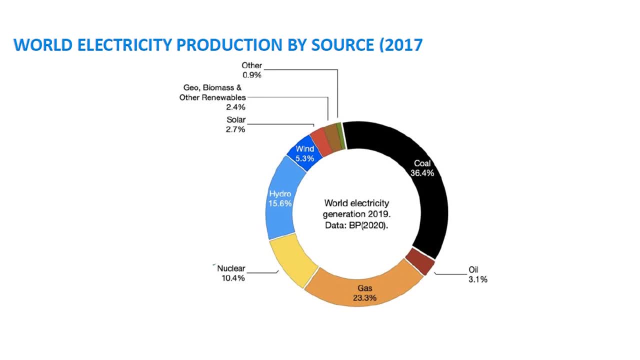 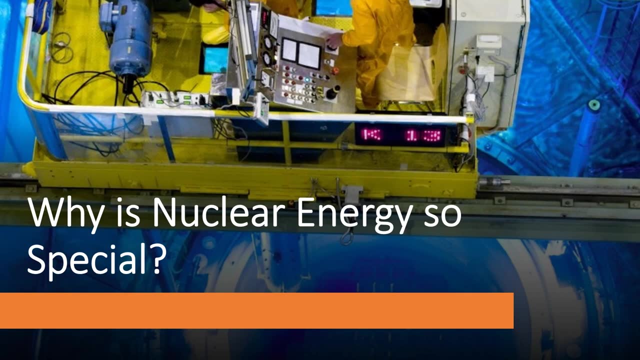 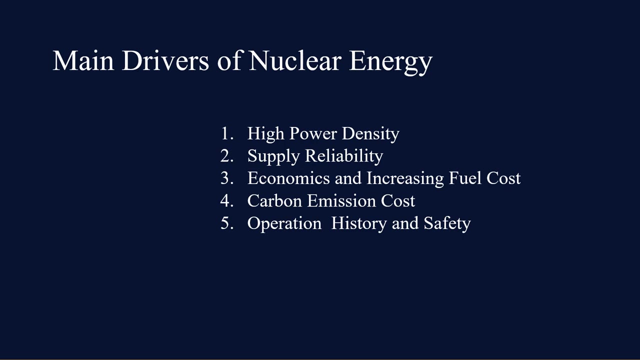 And only 2.7% of this is in solar energy. So why is nuclear energy so special? Well, there are two reasons. The first one is that it's very expensive. These are the main drivers of your nuclear energy. that makes it so special. 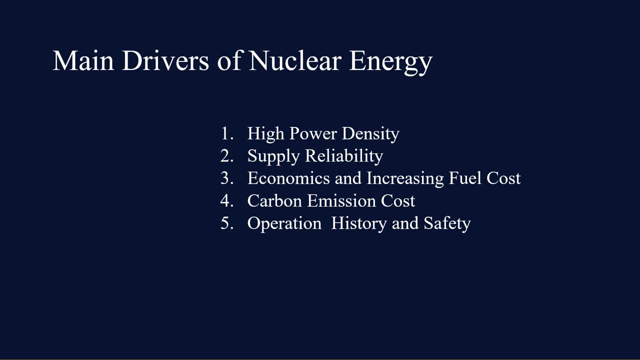 One is you have high power density. Second is you have supply reliability And then, of course, in economics, and increasing fuel costs and your carbon emission cost and on your operational history and safety. So we're going to discuss this one one by one. 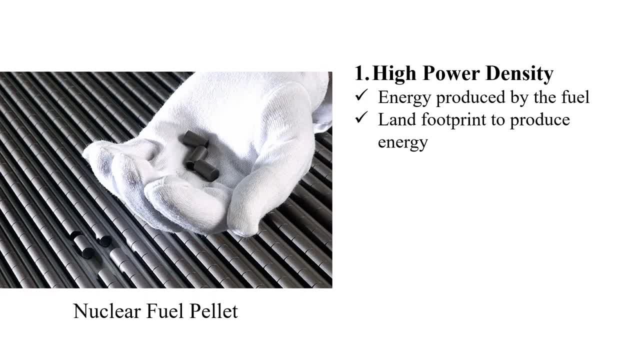 First let's talk about your high power density. And the main drivers of your nuclear energy are the energy consumption, And we're going to discuss this one one by one. First, let's talk about your high power density. First let's talk about your high power density. 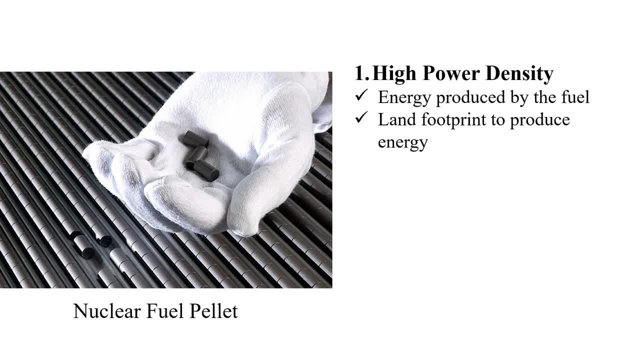 So what you see in the image is a nuclear fuel pellet which is actually very small And because of this one, you have a high power density, which you will see later why. And you have- let's talk about the energy produced by this fuel and the land footprint to produce this energy. 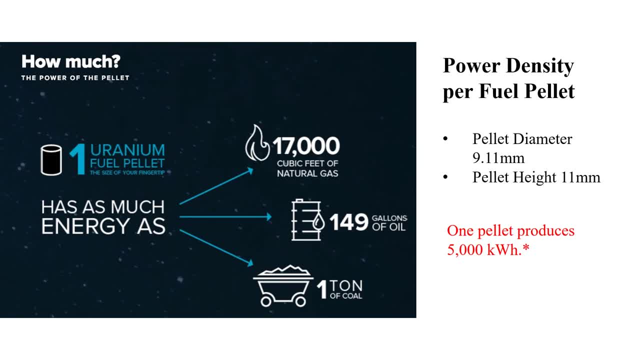 So your uranium fuel pellet is just 9.11 millimeter in diameter and it was a height of 11 millimeter. It is very small, but one pellet can actually produce 5% kilowatt per hour of energy, enough to power one town. 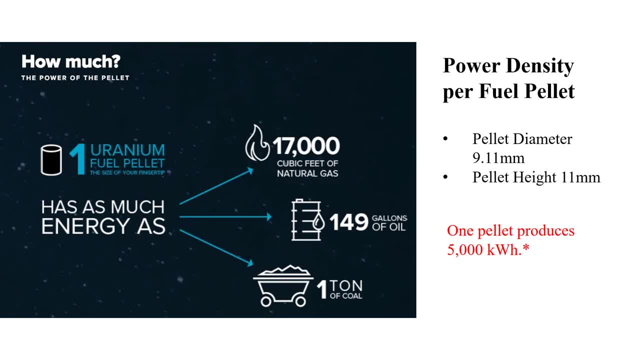 So one uranium fuel pellet has as much energy as 17 times 17,000 cubic feet of natural gas, has an energy of 149 gallons of oil and has an energy equal to one ton of coal, which is a lot. You're going to compare your one pellet of your uranium: compare it to 17,000 cubic feet of natural gas, 149 gallons of oil, one ton of coal. 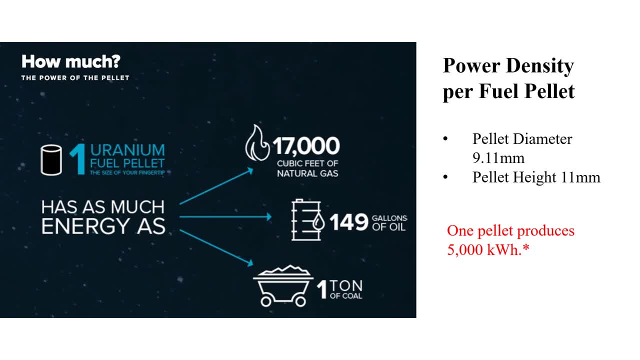 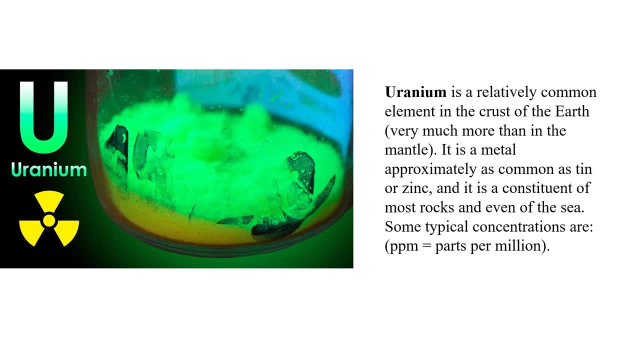 It's very much varied. It's very efficient as compared to the other sources of your energy, So the fuel that is mostly used is your uranium, which is a relatively common element in the crust of earth, very much more than in the mantle. 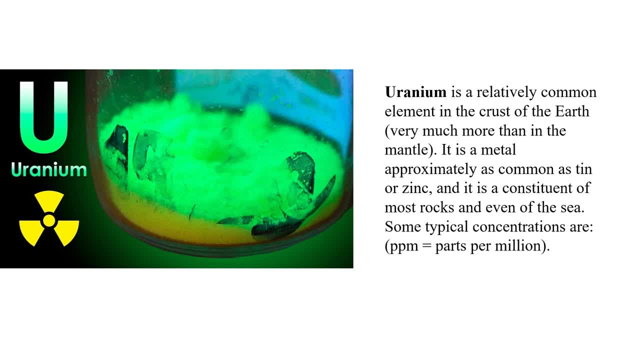 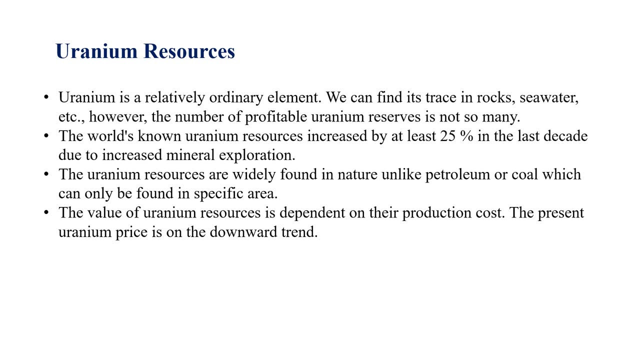 It is metal approximately as common as tin and zinc, and it is a constituent of most rocks and even at the sea. Some typical concentrations are in parts per million. So again, uranium is a relatively ordinary element. You can find its race in rocks, sea water, etc. 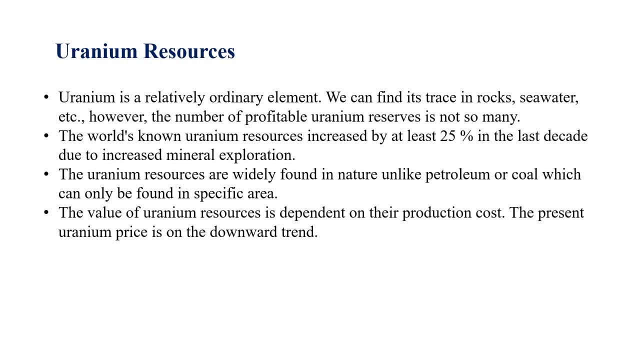 However, the number of reputable uranium reserves is not so many. The world's known uranium resources increase by at least 25% in the last decade due to increase in mineral exploration. The uranium resources are widely found in nature, unlike your petroleum or your coal, which can only be found in specific area. 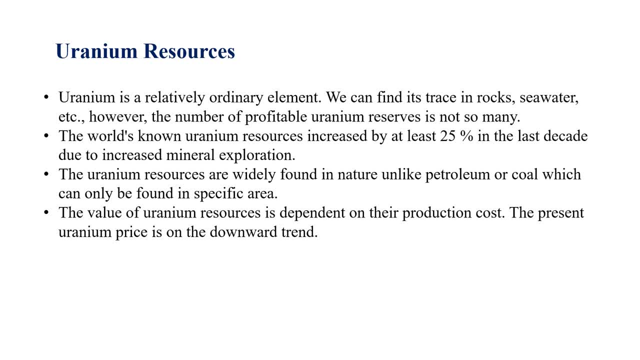 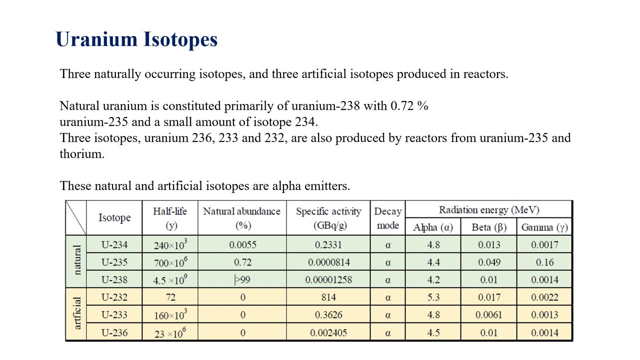 The value of uranium resources is. the value of the amount of uranium that is produced is dependent on their production production cost and at present the present uranium price is on the downward trend. we have three naturally occurring isotopes and three artificial isotopes produced in your reactors. natural uranium is constituted primarily of: 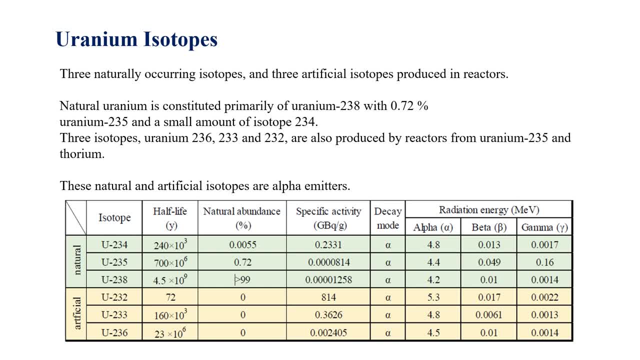 uranium-238, with 0.72% uranium-235 and a small amount of isotope 234.. Three isotopes of uranium- uranium-236,, 233, and 232- are also produced by reactors from uranium-235 and thorium. These are the natural and 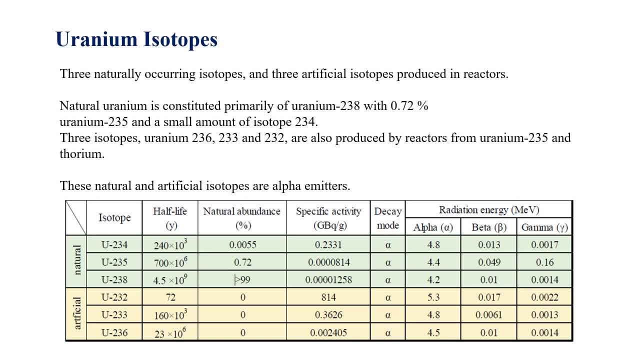 artificial isotopes, which are your alpha emitters. So again, your natural isotopes are uranium-234, uranium-235, and uranium-238.. And your artificial are uranium-232, uranium-235 and uranium-238.. 2,, 2,, 3, 3, and 2, 3, 6.. 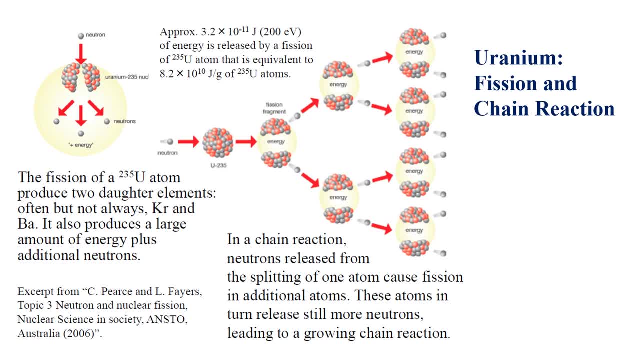 So again uranium. this is the fission and chain reaction for your uranium. We have already discussed this one earlier. The fission of uranium-2,, 3, 5 atom produce two daughter elements: often, but not always, your krypton and barium. 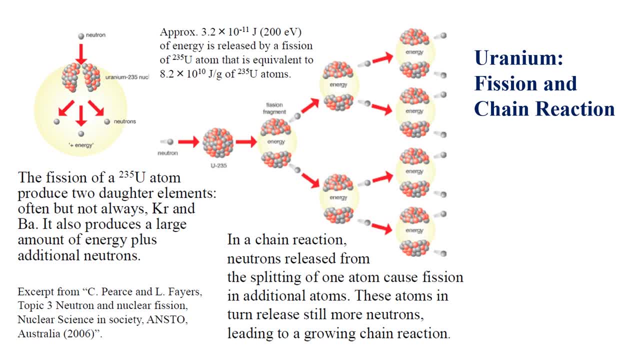 and it also produces a large amount of energy plus additional neutrons, creating a chain reaction. Your neutrons release from the spitting of one atom plus fission in additional atoms, So as you can see here, which creates the chain, but these atoms internally still more neutrons. 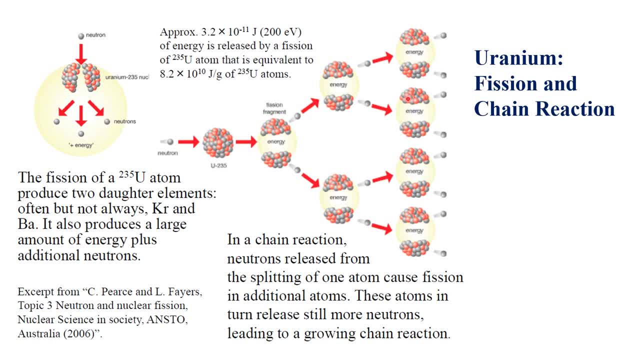 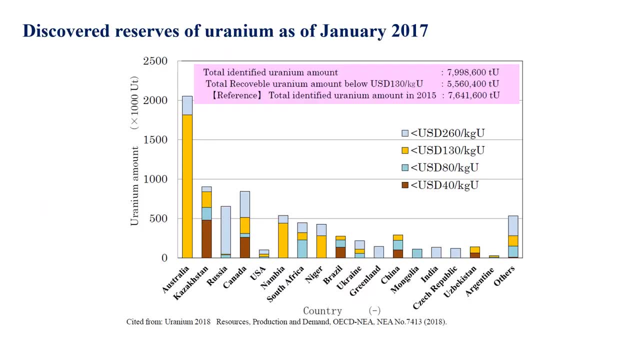 leading to a growing chain reaction releasing more energy in the process. This already discussed. So we have a lot of reserves of uranium as of January 2017.. So we have a lot of reserves in Australia, in Kazakhstan and in Russia. 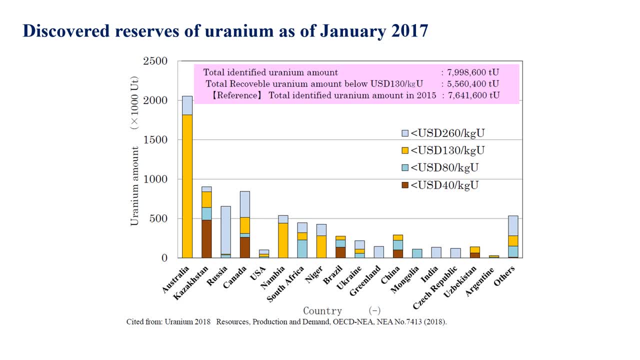 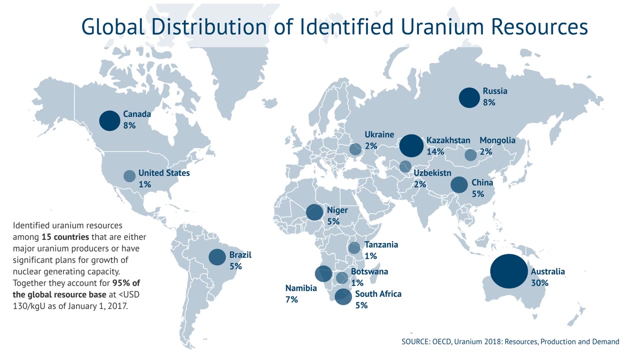 We also have some in South Africa, in China, in Mongolia and in India. So there, as you can see, uranium is very much available In many areas, unlike your coal and your fossil fuels in your natural gases. These are the identified uranium sources among 15 countries that are either major uranium producers. 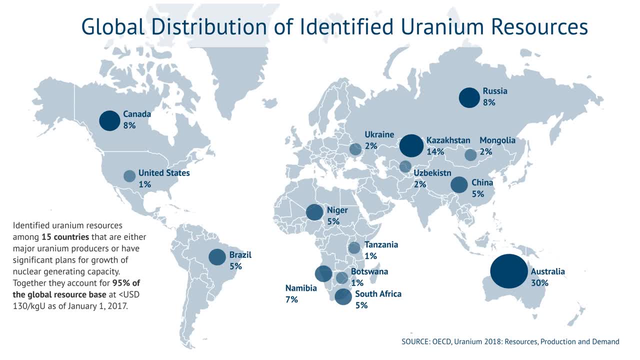 or have significant plans for the growth of the nuclear generating capacity. 30% of your uranium sources, of our uranium sources, are found in Australia And we have 14% of uranium sources in the United States. 49% of uranium sources are in the United States. 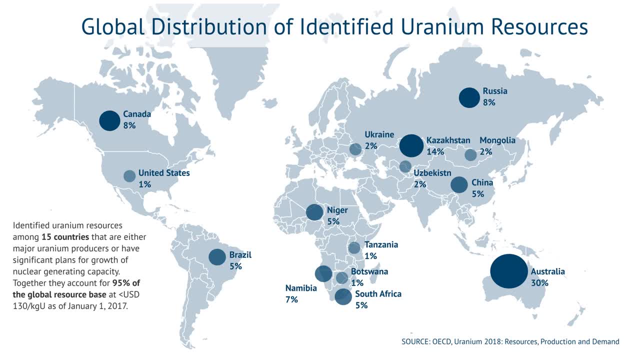 42% of uranium sources are in the United States, And the rest are spread out in the other parts of the globe. Of course, there may still be other areas which are still undiscovered, But, as you can see, your uranium sources is spread out evenly across the globe. 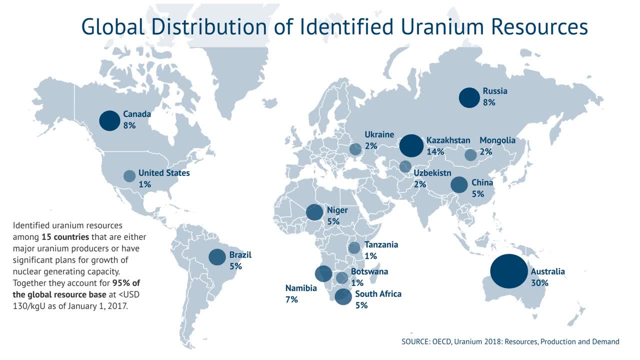 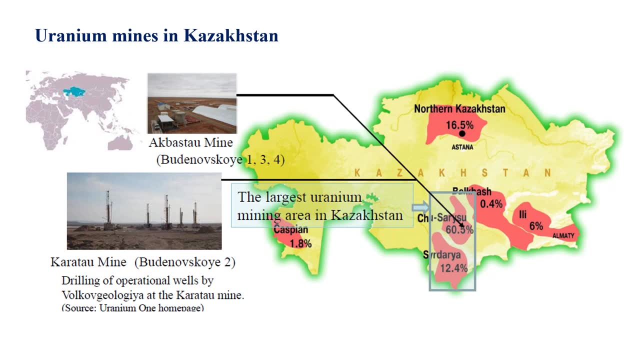 unlike, again, your fossil fuels or your natural gases. we have a uranium mine in Kazakhstan, so it's the largest uranium mining area in Kazakhstan, in Akbastal mine, and we also have a mine in Krakow mine. we also have uranium mines in Chusarisu and Sirdarya uranium province. 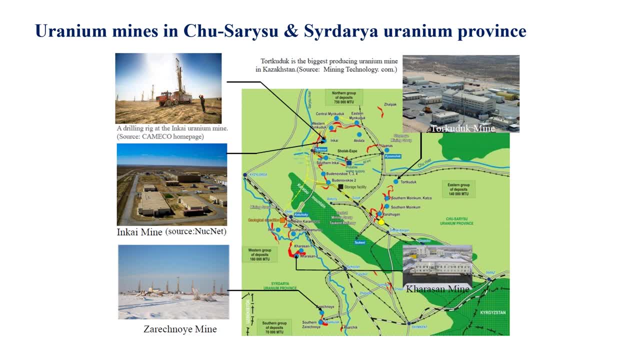 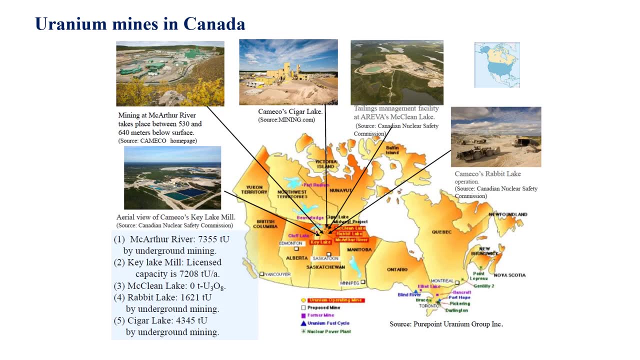 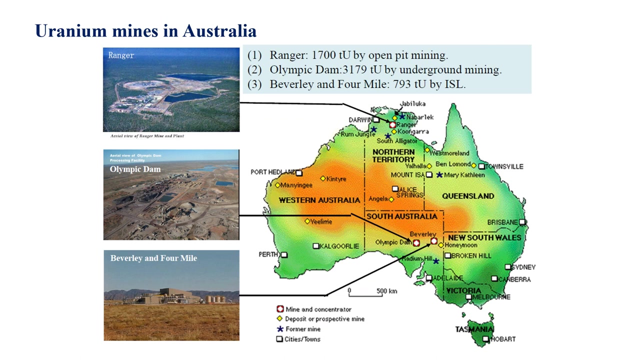 these are still found in Kazakhstan. so Kazakhstan is really a uranium mining province, as you can see. we also have uranium mines in Canada, mining at the MacArthur River in the Kamikos Sigger Lake. we also have uranium mines in Australia, the largest source of uranium. 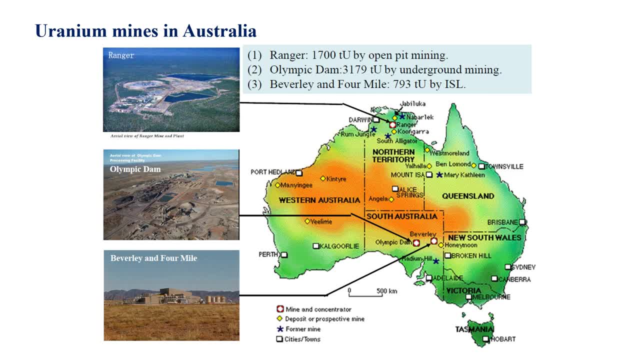 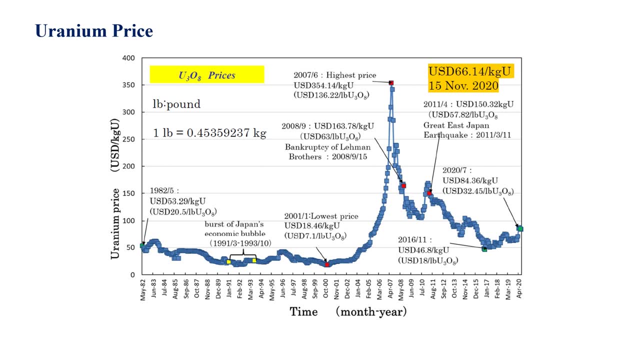 that uranium often extract, or loyal uranium, around the world. this is the uranium price. throughout the years there was just a steady increase in the price around around 2005 to 2007, where at 2007 you have the highest price of 354 US dollars per kilogram of uranium. 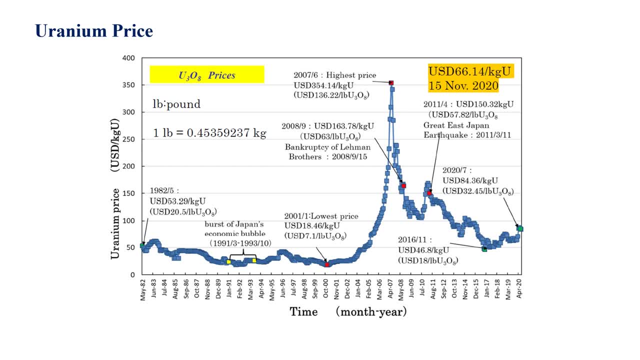 but after 2007, there was already a downward trend in the price of your uranium up to 84.36 US dollars around on on 2020. okay, and the lowest price now is just around 66.14 US dollars per kilogram of uranium, which is the price last November, 15 of 2020. 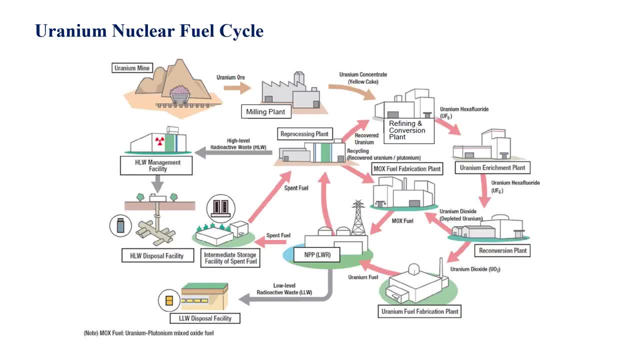 so this is your uranium nuclear fuel cycle. it starts in your uranium mine and then which, where you can get your uranium or your uranium ore, and from that it goes to the, the milling plant, and then your uranium concentrate, which is a yellow cake, will be refined and converted in your refining. 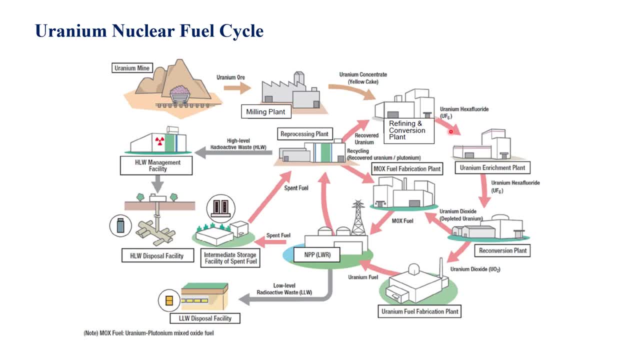 and conversion plant and then from this start the process of your uranium hexafluoride and then up to your uranium enrichment, up to the reconversion plant, uranium field propagation, and it goes around until it's used in your, in your power plant and you also can pay on. 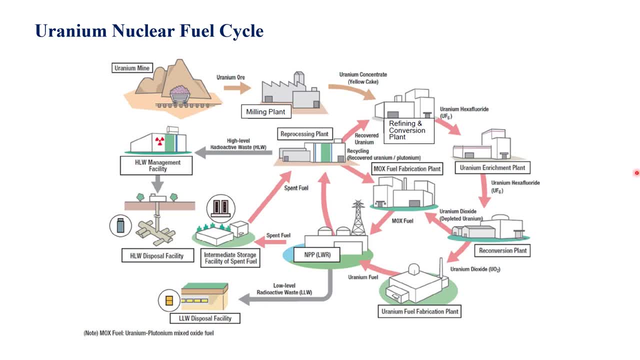 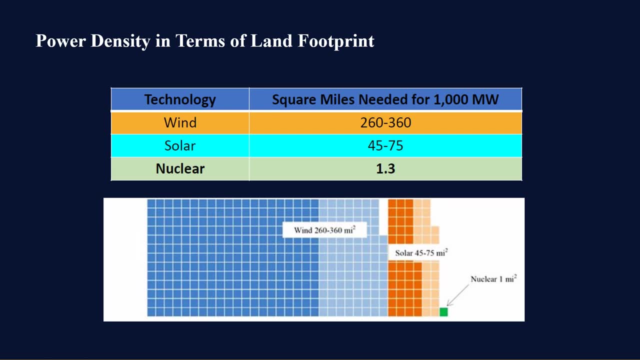 also have your disposal facility, of course. let's talk about the power density in terms of land footprint. let's compare your wind, your solar and then your nuclear, and, as you can see, um, for your wind, you need 260 to 360 square miles for 1000 megawatts of energy, and for your solar, you need 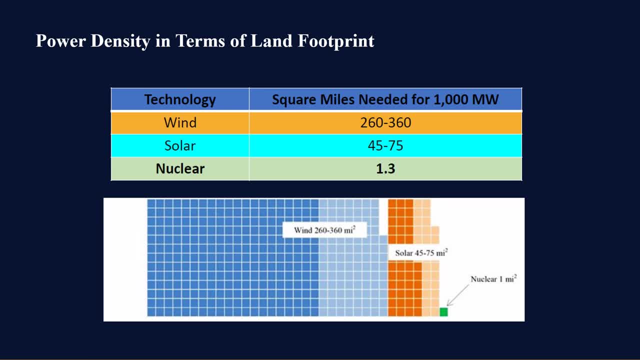 around 45 to 75 square miles for just 100 megawatts of electricity. but for your nuclear, you only need 1.3 square miles for 1000 megawatts of energy. this can be seen here in comparison. this is the square mass needed for your wind. okay, this is for your solar, and then this is for your nuclear. 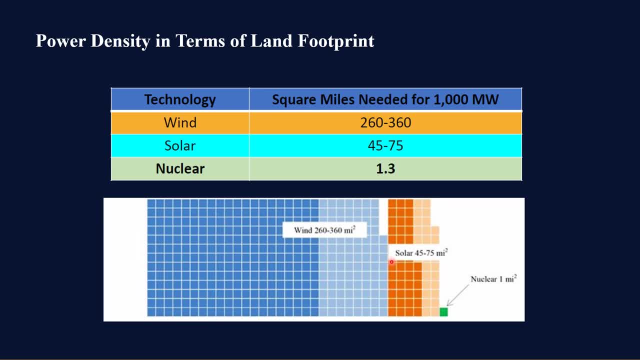 compared to the wind and the solar. your nuclear only takes a very small area of land to produce 1000 megawatts of electricity and if you can remember your wind and then your solar, actually small sources of, or it can only produce small amounts of energy. 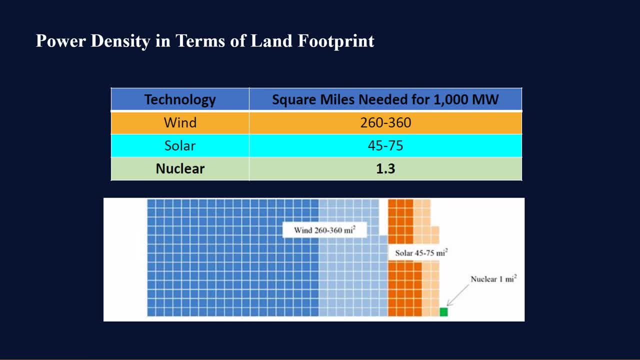 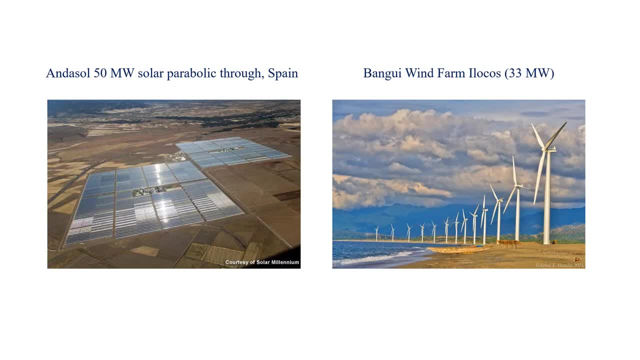 that's why you need larger plants or larger areas for this one to produce 1000 megawatts of electricity. okay, this is the power you will use. just in comparison, you have here your anda sol 50 megawatt solar power parabolic flow in spain. so it it really, uh, takes up a lot of space. and this is the bungie. 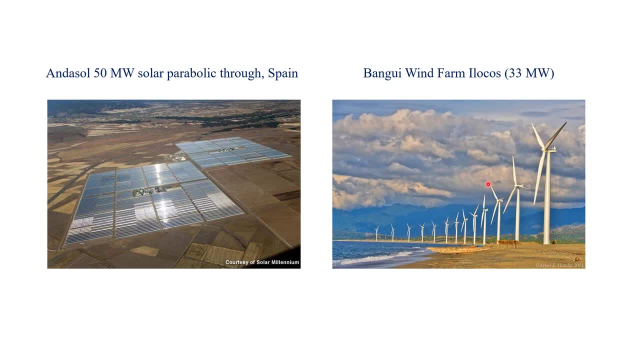 wind farm in Ilocos which can produce 30 megawatts of electricity. so you can produce 33 megawatts, but, as you can see, you're your. your main goal is to use 50 megawatts of solar energy. your, your, your wind farm can actually take up a lot of space. so, as you can see, here it takes. 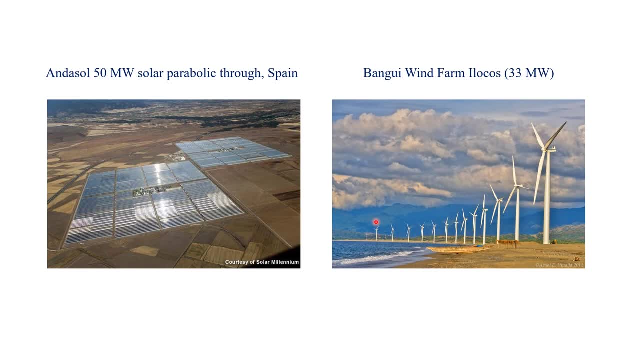 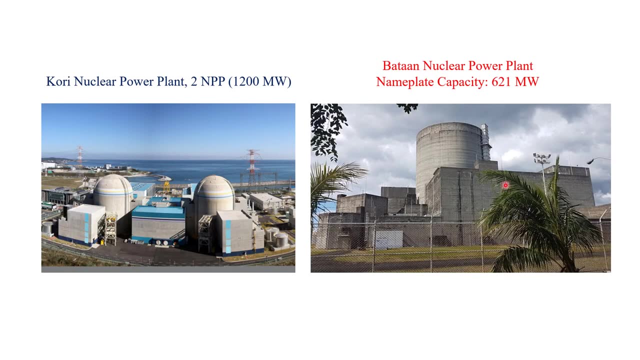 uh, mostly the shoreline of your, of your, of your ocean. compare it with your power plants, say, for example, for your core nuclear power plant. so this is just a very small area, but it can. it can reduce around 1200 megawatts. if the Bataan nuclear power plant was commissioned, it has an intake capacity of 621 megawatts. this 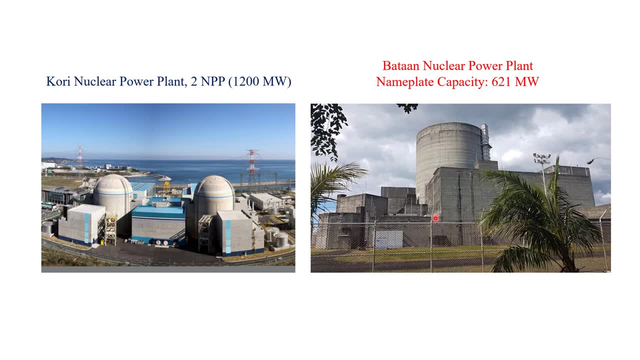 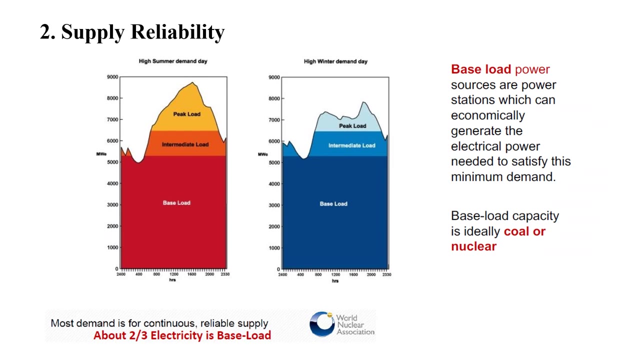 is just a very small area compared to Bangui uh wind farm, but this can produce a lot more energy than the one in uh Ilocos. now let's talk about the main, the next main driver of your nuclear energy: the supply reliability. most demand of electricity is for continuous, reliable supply. 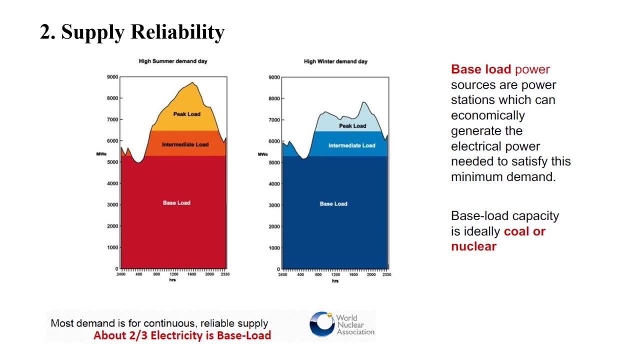 and about two-thirds of electricity is baseload. what is baseload? baseload power sources are power stations which can economically generate the electrical power needed to satisfy this minimum energy supply demand. baseload capacity is ideally coal or nuclear. this is the baseload, or the power demand. 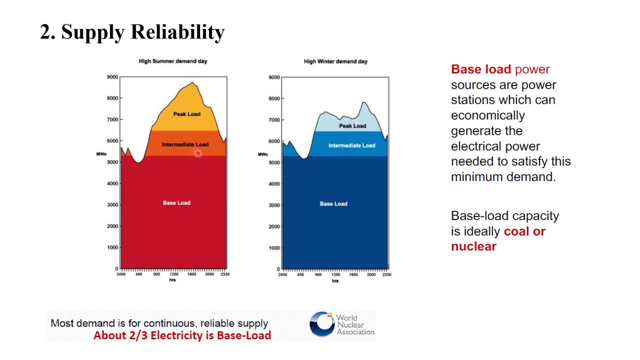 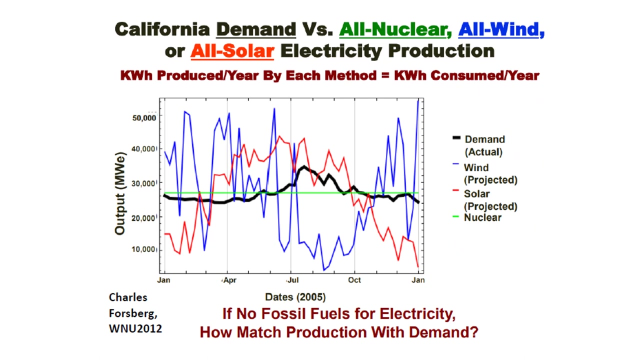 during summer in in areas which can experience summer and winter. so there is really a peak load, a very big peak load, especially in summer and below here. this is the baseload that needs to be continuously uh supplied, and only two allergenic sources of electricity can continuously. exactly, doc. 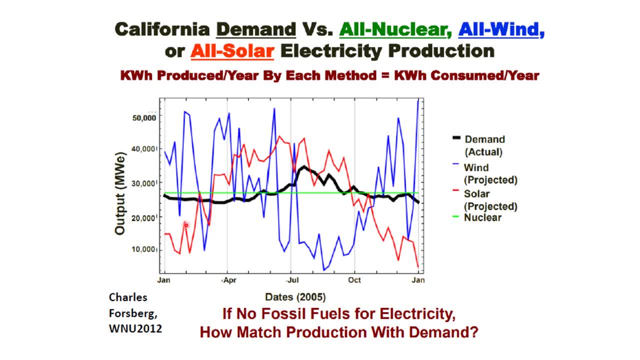 supply your base load and this is your coal and nuclear. as you see here this is the California demand of California demand vs all nuclear, all wind and all solar electricity production. so the black line here this is your California demand for electricity. there are there are several different fuel sources and bamboos are used and energy in 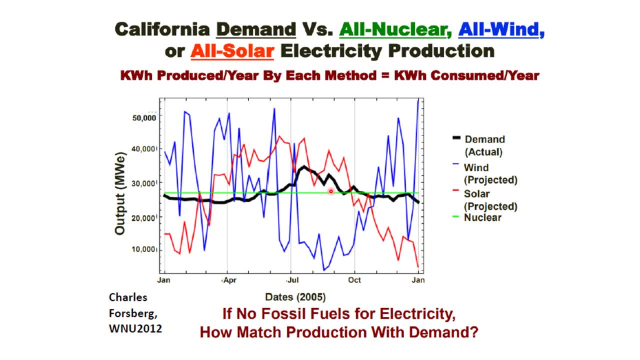 green one is for all nuclear, the blue is for all wind and then the red is for your all solar electricity production. as you can see, if you compare your demand with your wind in blue, there is a very big fluctuation in the base load output or the energy output in your wind energy. 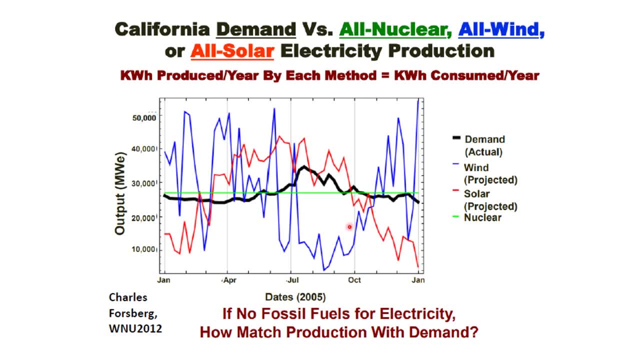 because it's not always that you have a, a windy weather. so there might be times wherein- uh, your, your, your wind energy cannot supply the, the base load and, comparing it with the solar, there's still a fluctuation, because there are, there is your daytime and then there is also your. 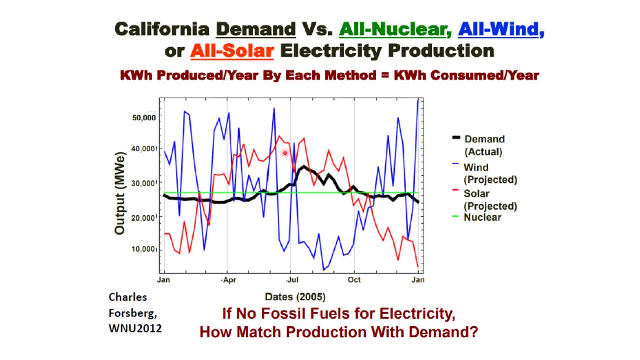 night time. of course, in the night time your base load will not be uh continuously supplied by your solar and only your nuclear. the green line can supply your uh, your base load demand, uh continuously and reliable uh with uh, uh great reality, reliability: if no fossil fuels for electricity, how much? 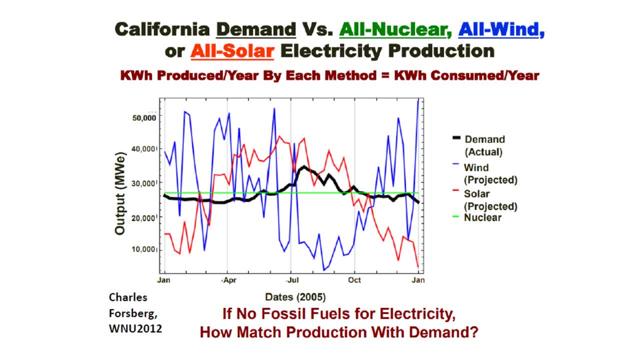 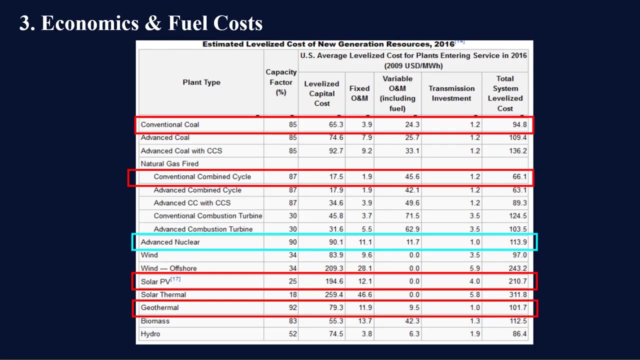 production. uh can satisfy this demand, so there will. there will be a very, very hard time uh supplying with only your wing and then your solar energy. the next main driver is your economics and fuel cost. uh, this is just a comparison of your uh estimated levelized cost of new generation sources in 2016.. uh, let's look at the capacity. 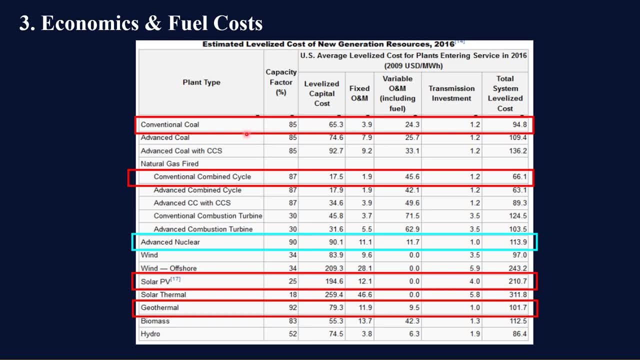 factor. so for your conventional coal the capacity factor is around 85 percent. for advanced nuclear you have 90 percent, for your solar only 25 and then for your geothermal you have 92. compared to the other uh sources or to the other plant types, there is really a great capacity factor for your advanced nuclear. however, 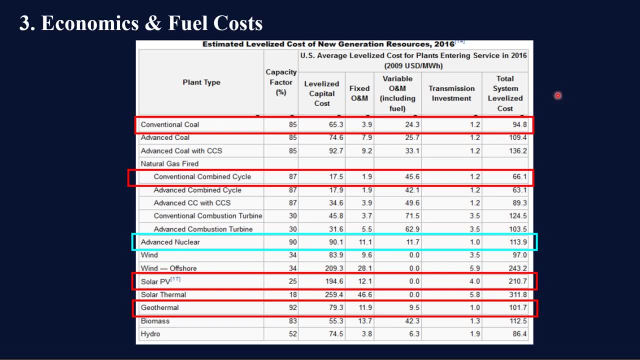 if we are going to compare the total system, levelized cost, the cost, the cost throughout the day and the cost of the solar is really really high compared to the conventional coal. the cost of the solar, which has been, is really high compared to the conventional coal. so, for example, your advanced nuclear is actually higher at 113.9, but it's not even compared to. 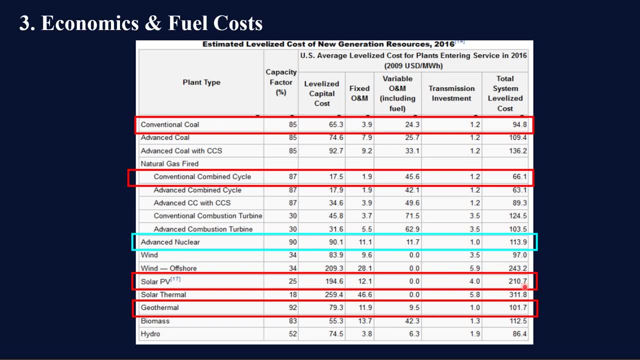 the solar. you are not even compared to the conventional coal, the property tax that's in maintaining and making um or establishing a power plant, um compared to than your nuclear power plant, um, your solar is around 210.7 but your advanced nuclear is just in the same level with your uh, your, your conventional coal and then even in your 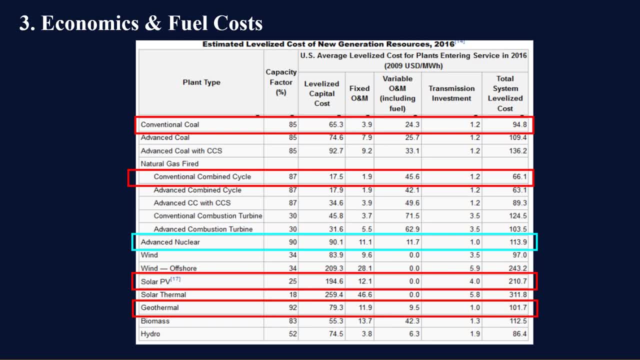 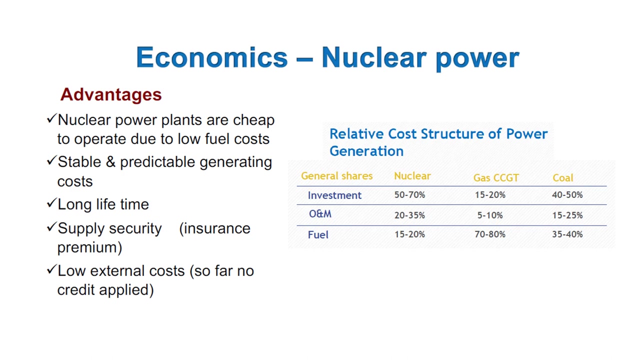 geothermal and then your uh, your biomass. so there is really a big difference in terms of the capacity factor and then the total system levelized cost in your nuclear uh, nuclear power plants, the advantages in terms of the economics for your nuclear power plant, nuclear power plants. 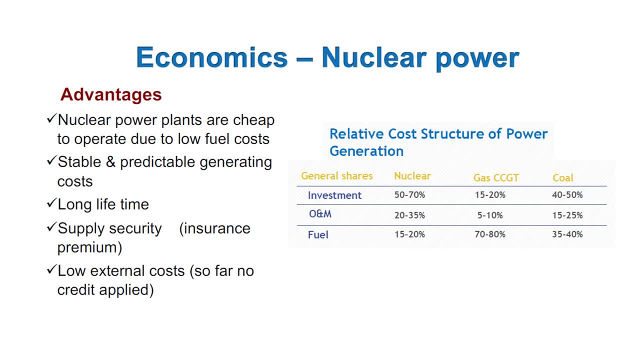 are cheap to operate due to low fuel costs. as you've said earlier, if you have one nuclear pellet, this is more cheaper as compared to tons of coal or gallons of your. your petroleum- and also its stable and predictable generating costs, compared to wind and solar, just a long lifetime. you have supply security and then low external. 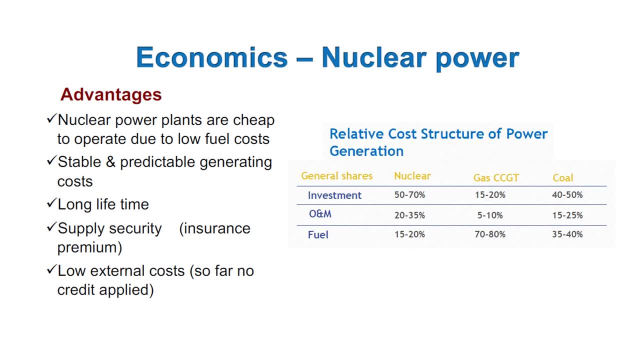 costs. so far, no credit applied and this is the relative cost structure of power generation for investment. um, if you're going to compare uh investment with nuclear gas and coal, you really need more investment when it comes to nuclear as compared to coal or your gas. it's because, um establishing a nuclear 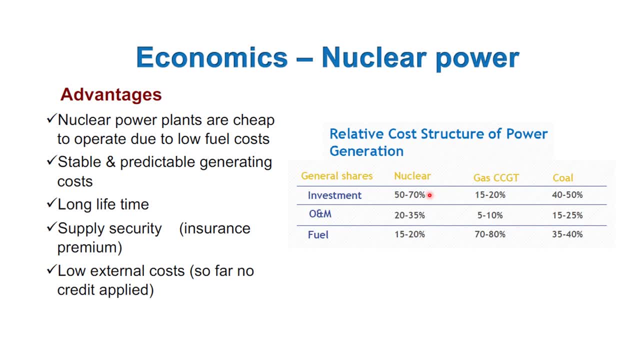 power plant will take up at least 10 years. you need to pay a lot of consultants, and then the making of the plant itself or the constructing of the plant itself will take long years, so you really need a lot of investments. but in the long run, though, you have a lot of investments in. 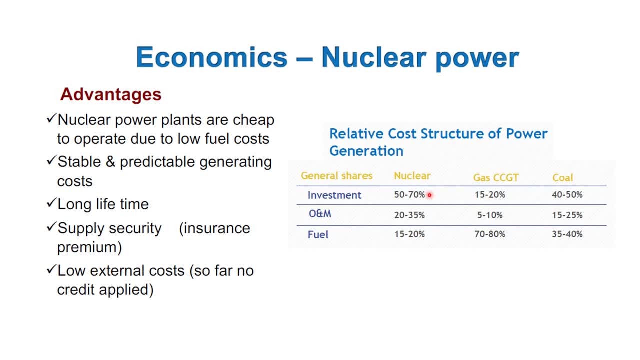 the beginning. you have a long lifetime for your power plants and, of course, it will be more cheaper to operate than compared to your coal and um your gas. as you can see, the fuel is 15 to 20% only, compared to the 35 to 40 percent operating uh cost in your your coal. 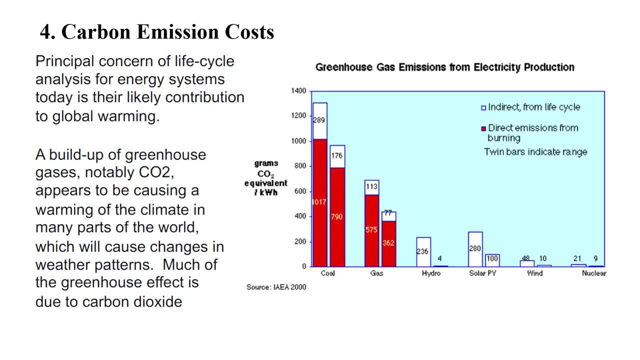 the next main driver that we're going to discuss is on the carbon emission cost. so you have principal concern of life cycle analysis for energy systems today, which is their likely contribution to global warming. it is a big concern nowadays, especially your power plants. that's why there are many rallies or many issues with coal power plants. 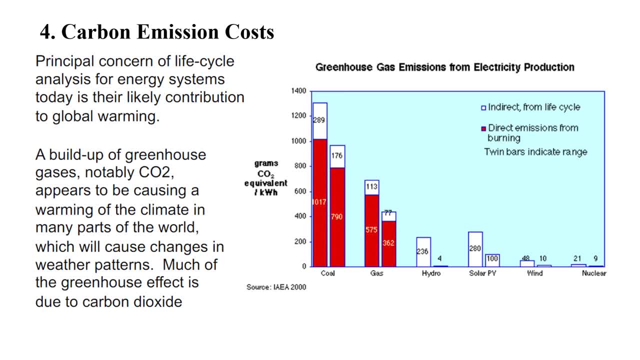 a build-up of a build-up of greenhouse gases, notably your carbon dioxide, appears to be causing a warming of the climate in many parts of the world, which will cause changes in weather patterns. much of the greenhouse effect is due to carbon dioxide, and these are the bar. 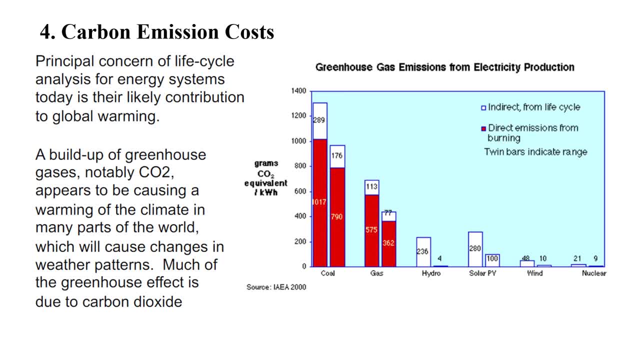 graphs of your greenhouse gas emissions from electricity production, comparing your coal, gas, hydro, solar, wind and nuclear. and as you can see, there is a high indirect um indirect emission of greenhouse gases in your coal also, your direct emissions are high direct emissions from burning also in your gas there's still a high direct emission. 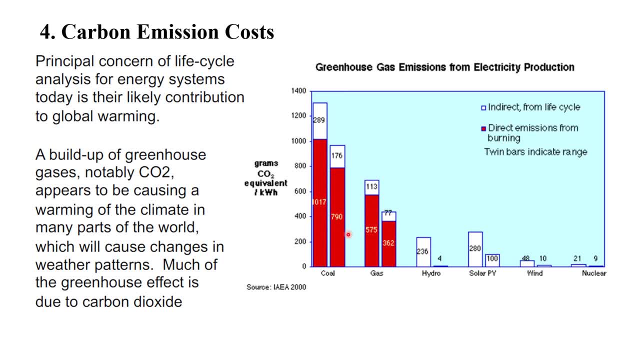 and comparing your coal and your gas with your nuclear, your nuclear energy is really feeling good. there's just a low um emission of greenhouse gases for electricity production in your nuclear compared to your to your core and then to your to your gas. so just around 21 and 9 indirect. 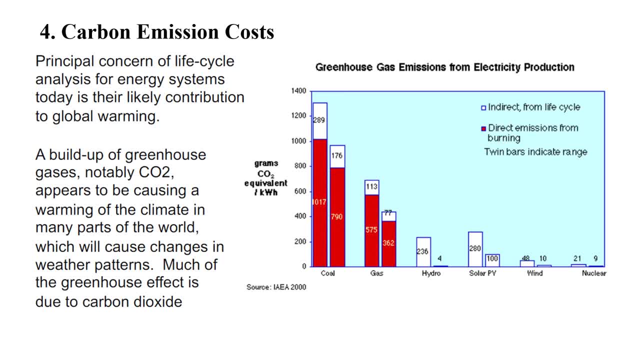 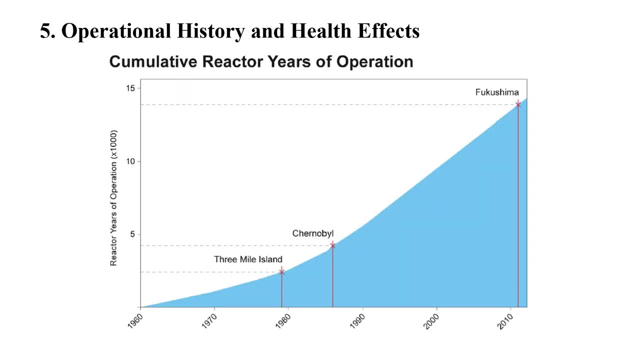 from the life cycle, and this one is just from, not from the uh, from the uh direct emission itself, but can be seen from uh, the mining of your uranium and and so on. so next year is your operational history and health effects. this is the cumulative reaction: years of operation. so you have your reactor, years of operation and these are the accidents. 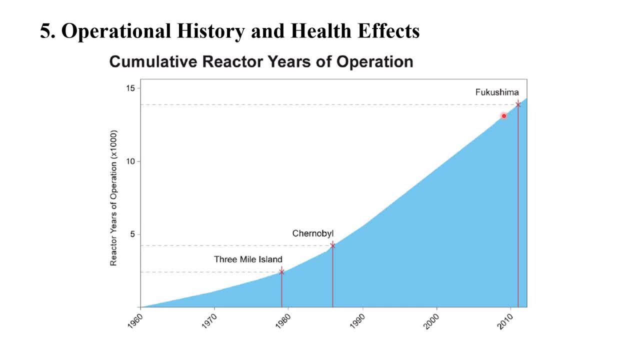 that had happened in the past years. since the start of the operations of nuclear power plants, there were just three accidents, without blends of things like Riverside and En Nokia System incidents that have caused large damages. One is the Three Mile Island power plant accident, and then you have your Chernobyl, which is one of the famous accidents in your nuclear 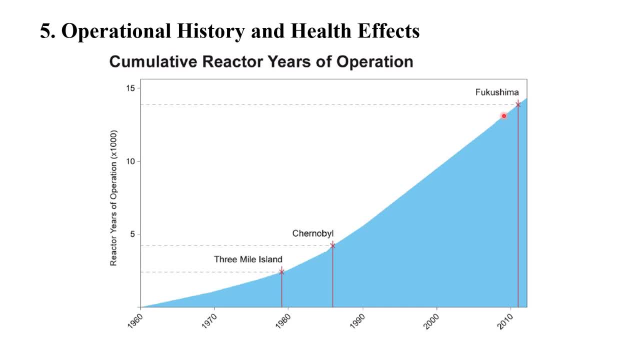 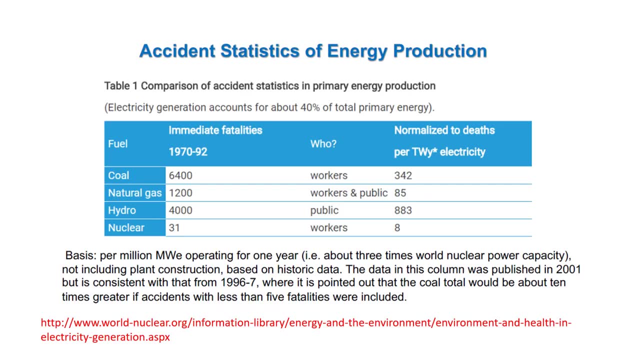 power plants. and then you have your Fukushima, which is very recent, which we have all seen. that happened in Japan. Comparing the accident statistics of energy production in coal- natural gas, hydro, nuclear- you see that from 1970 to 1992, we actually have 6400 immediate fatalities in coal: 1200. 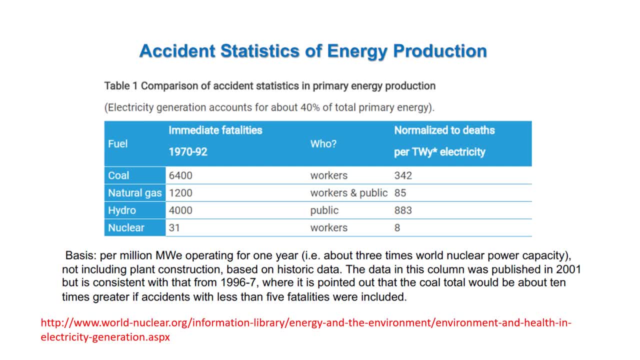 immediate fatalities in natural gas and 400 immediate fatalities in your hydro power plants, But we only have 31.. Fatalities in your nuclear power plants, and mostly in the coal- you have your workers of 342 normalized deaths per terawatt year of electricity- and then in your natural gas. 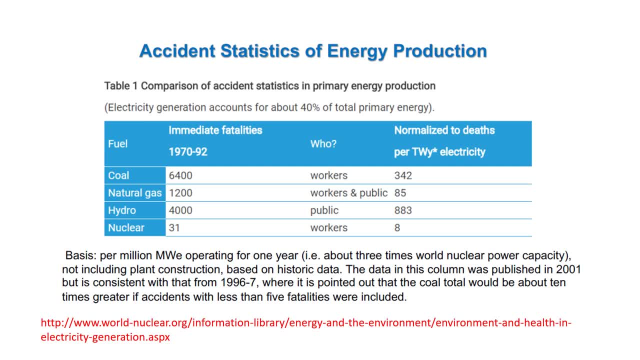 it involves your workers and your public For your hydro. it involves the public because, as you can see, when your hydro thermal plants broke out, The water, The water, is released to the neighboring town, So there will be more deaths from that as compared to the eight workers in your nuclear. 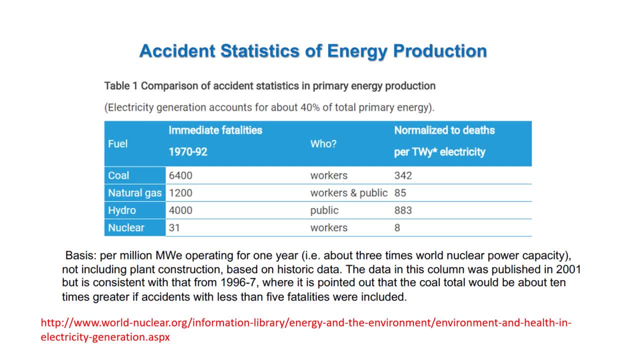 power plants. So the basis for this one is per million megawatt electric operating for one year And, as you can see, nuclear is actually not really that dangerous compared to coal, natural gas and hydro. But we're very much in fear of nuclear. 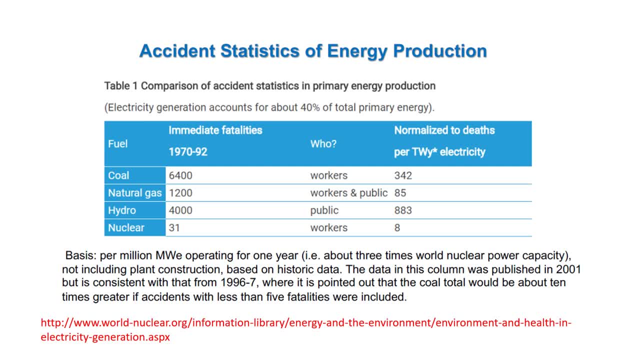 But we're very much in fear of nuclear. But we're very much in fear of nuclear, And this is just because of the three accidents: your three-mile island accident, your Chernobyl accident and then your Fukushima accident. What we're pairing here is the radiation. 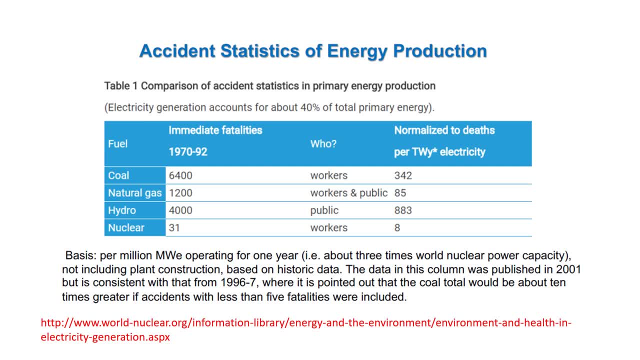 But we have already discussed in the previous lessons that radiation can actually be prevented if you use the right instruments and you follow the right protocols. So, in summary, this is from this comparison here: Coal particles and energy. So, in summary, this is from this comparison here. 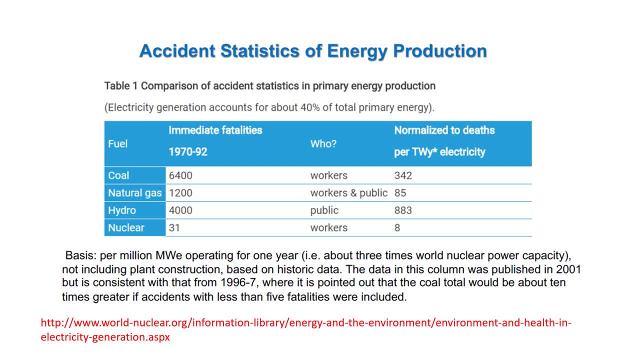 Coal particles and energy. So, in summary, this is from this comparison here: Coal particles and energy. So you have to take into account that most nuclear power plants actually have more deaths. compared to your nuclear power plants, Your coal is actually more dangerous. 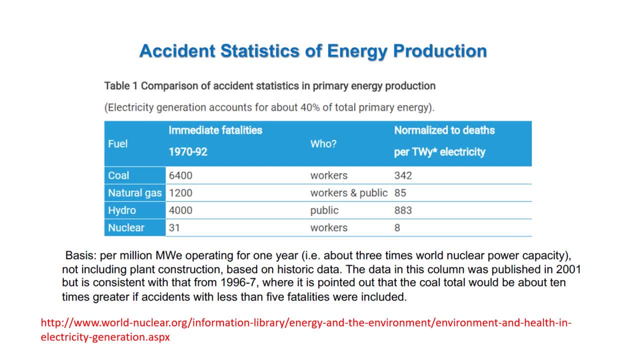 Your coal is actually more dangerous, But it's also going to have positive impacts on your recent4 natural gas commitments And, of course, this goes to step to step. coals are going to bring more greenhouse gases, So why do you fear your nuclear power plants? 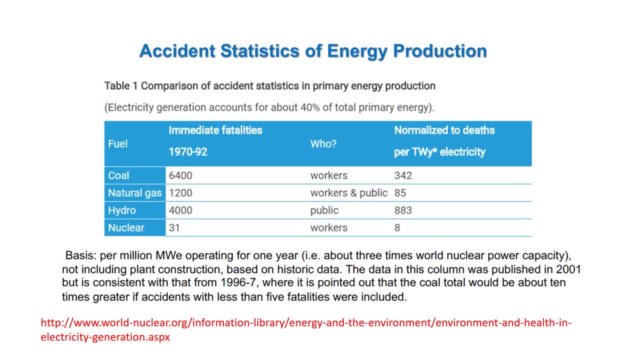 So why do you actually fear your nuclear power plants, Despite the main drivers of your nuclear energy that we have discussed in the previous sessions, despite the main drivers of your nuclear energy that we have discussed in the previous sessions s 그다음에, we also look at the replaceable. 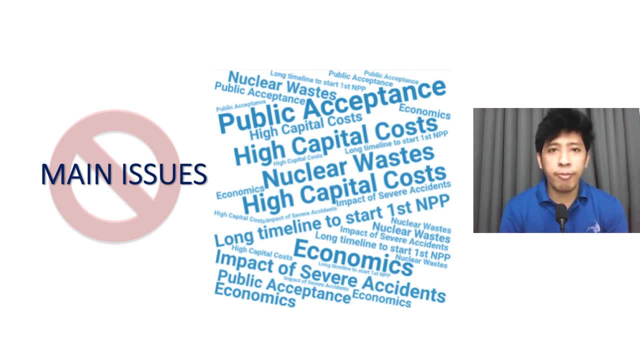 s livestock demand is on the mark in nuclear power plants, especially from diesel near gas. Arai, Arai, Arai. nuclear energy that we have discussed in the previous sections. there are still many issues about nuclear energy. that makes it hard to enter into the. 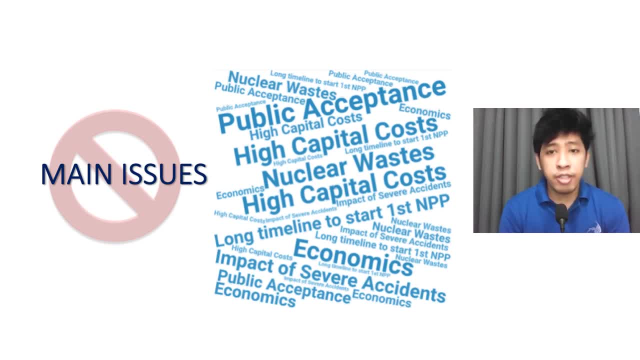 Philippine setting. so, as you can see, we are just one of the countries which do not have a nuclear power reactor yet, and these are because of the following issues: first, you have your public acceptance. I think one of the reason or the main reason why your Bataan nuclear power plant was not fueled up is because 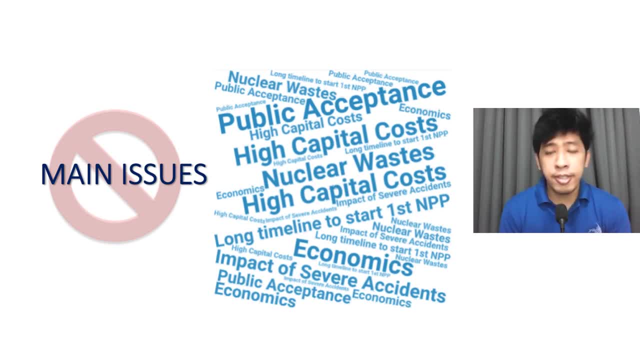 it happened during 1986, wherein, in April 1986, you have your Chernobyl accident and, if you can remember, President Marcos was ousted from from presidency because of people power in February of 1986 and by April 1986, it was now Cory Aquino who is in. 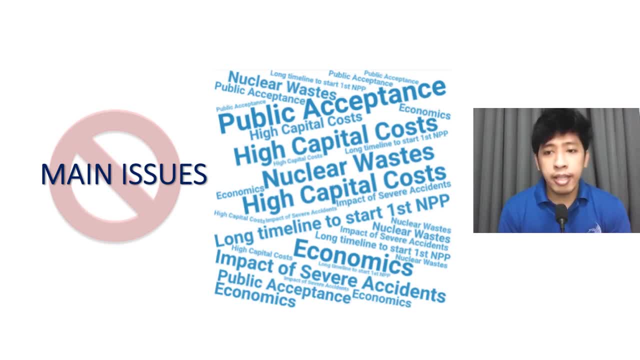 uh in office and her government decided not to fuel up the Bataan nuclear power plant following the nuclear accident in your Chernobyl. so if you're going to ask many nuclear engineers or nuclear scientists, one of the reasons why the Bataan nuclear power plant was not fueled up or was not commissioned was 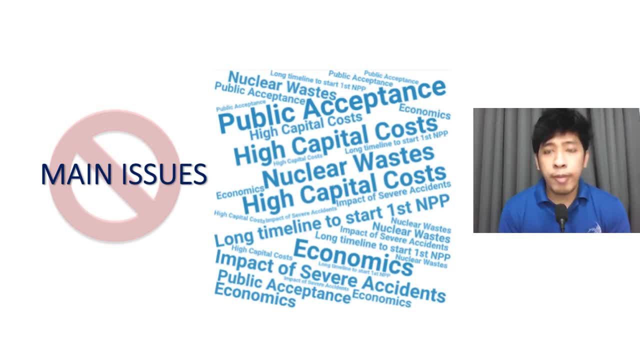 because of the Chernobyl accident. so there is a low public acceptance because the Filipinos feared that. the Filipinos feared that this may cause a lot of problems in the future. also, another reason is that there was an issue with the structure of the Bataan nuclear power plant. the Filipinos 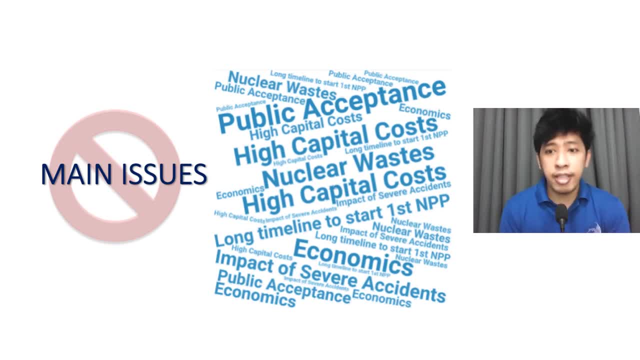 feared that in one day this might create some accident, just like the the Chernobyl incident. another thing is: after the Bataan nuclear power plants, there was no no other plans to to construct another one here in our country. it's because of the high capital cost. one power plant can take up to 10 years to construct, and the shortest 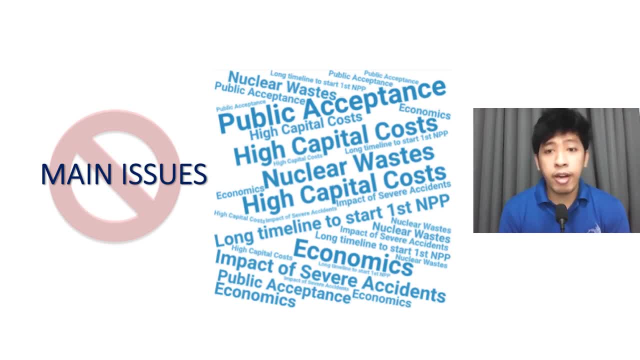 construction of your power plant was done in the United Arab Emirates, so they took them only seven years. but remember that you- UAE- is a rich country, so they have a lot of money to pay for consultants. they have lots of money to pay for consultants and they have a lot. 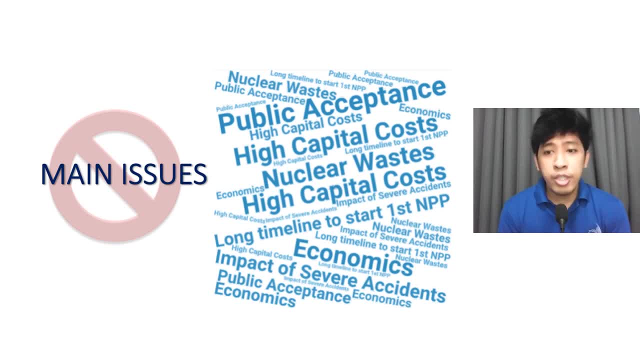 a lot of money to pay for consultants and they have a lot of money to pay for consultants, of money to to speed up the construction process, which is what we lack here in the philippines. another issue is you have your nuclear waste. it's still, which is still, an issue here. 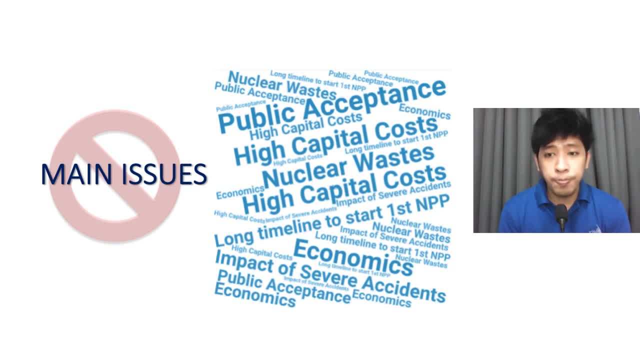 or an issue now all around, all around the world. um, your nuclear waste is used to be, um, uh, how do you call this? it's used to be, uh, thrown into the oceans. no, but now there are other plans to construct um waste facilities, but so far most of the waste facilities are not yet in in working. 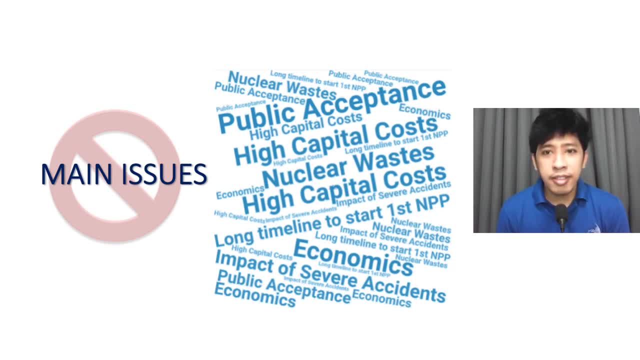 and um, also, you have your long timeline to start, uh, the first nuclear power plant. that's also another reason, and so far, those are the reasons, the main issues, why it it takes so much time to commission order to construct a power plant, especially here in our country. 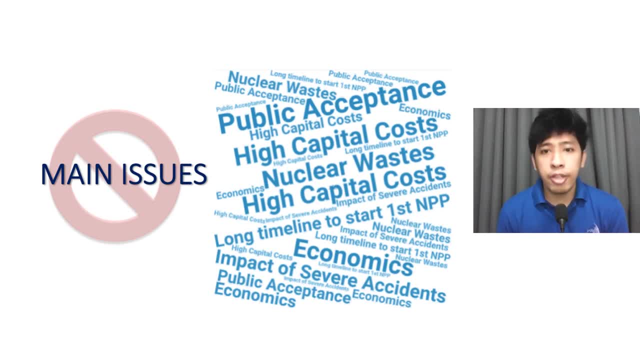 so you have your public acceptance, your high capital cost, your nuclear waste and a long timeline to start your first nuclear power plant. you.